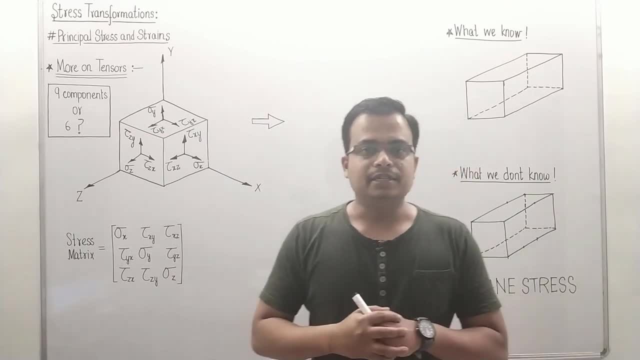 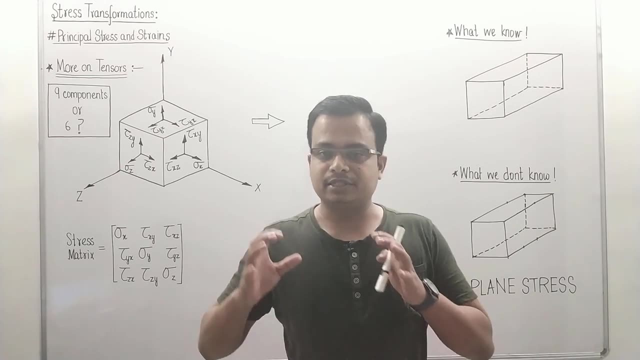 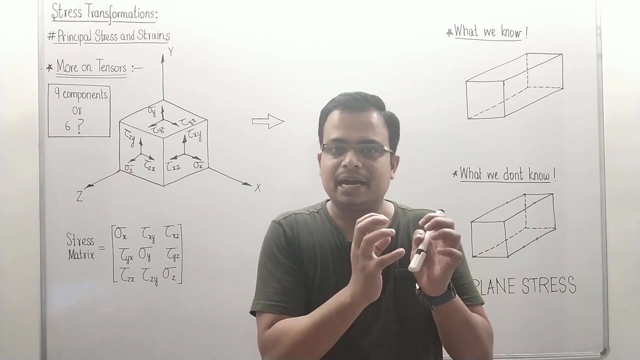 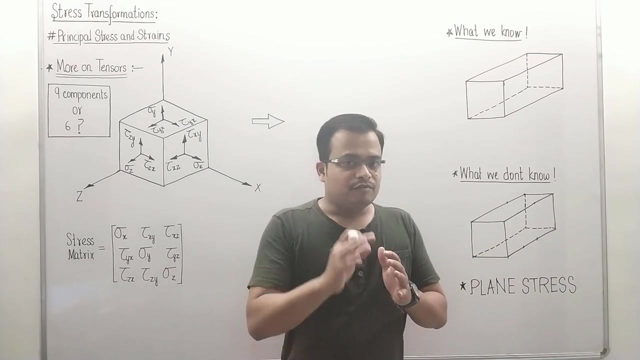 Hello everyone, this is Manas, your friend and tutor, And guys, I'm back with another video on mechanics of solids. The topic for today, or rather the chapter, is going to be stress transformations, principal stress and strain, something which is also referred to as compound stress and strain. Now, before we start talking about as to what we are going to learn in this particular chapter, we first need to touch upon a basic concept of a tensor. Now, guys, 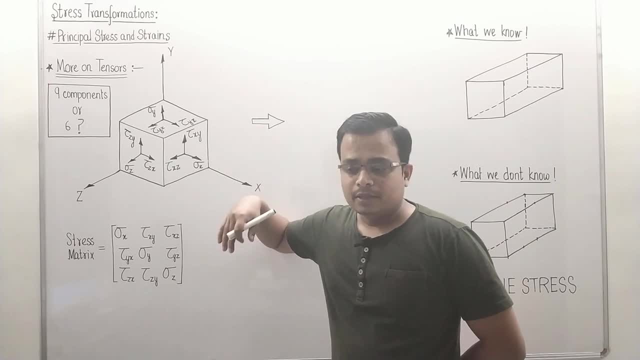 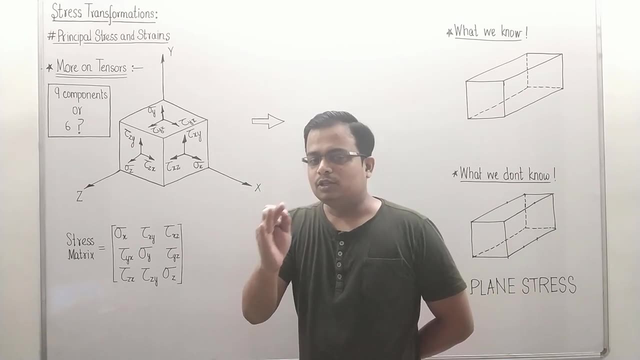 until now. the one thing that we're absolutely sure about is that a point inside a rigid body is subjected to, or is characterized by, six normal and shear stress components. Did I just say six? Wasn't it supposed to be nine? If you just try to make a count of the total number of different components of stress, it works out as nine, isn't it? So what is the answer? What is the right value? Is it nine component or six? If you ask me? 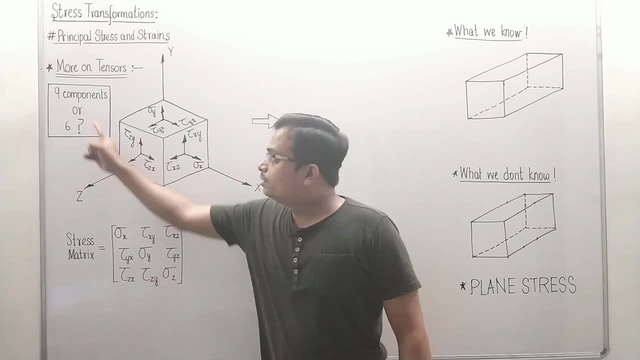 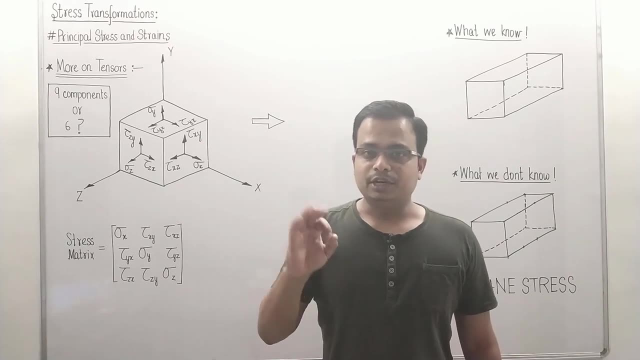 well, both of them are correct. If we just try to make a count, then that will work out as nine, But effectively there are only six components of stress. three of them are normal stress components and the remaining three are shear stress components. Well, that can essentially be worked out with the help of this three dimensional state of stress at a point inside a rigid body which is subjected to external loadings. Now just take a look at this. 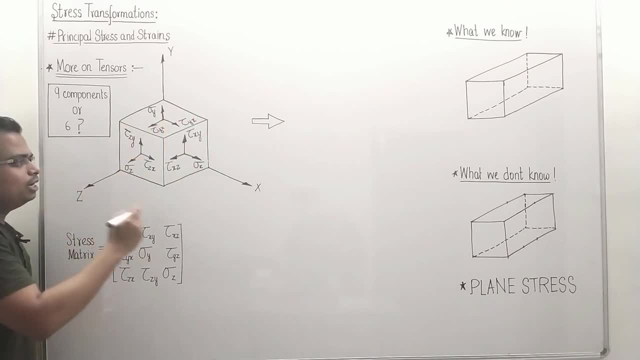 This, this element over here, small element, is acted upon by nine different kinds of stress, isn't it? And if you take a careful look, this is tau x y And this over here is tau y x. Well, to tell you, these, both shear stresses are equal in magnitude. but I'll prove it to you right now. And if you watch, if we just try to have a look at this entire arrangement from this side, from the 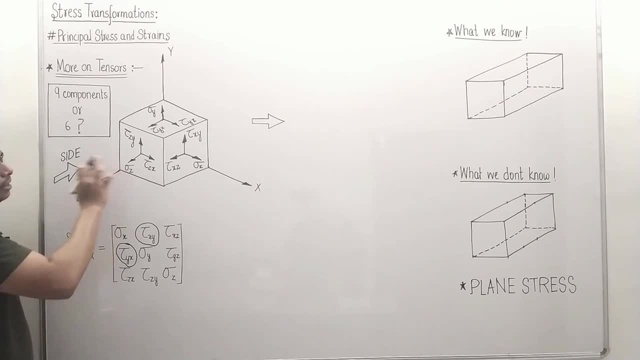 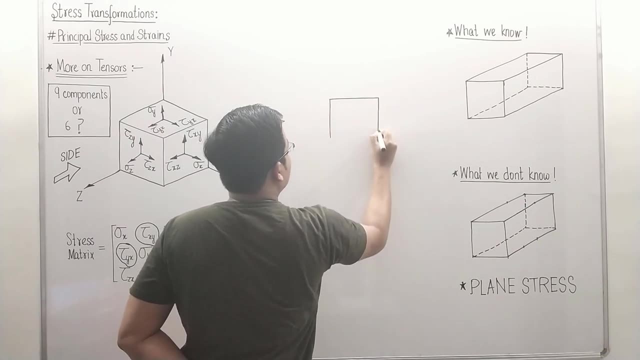 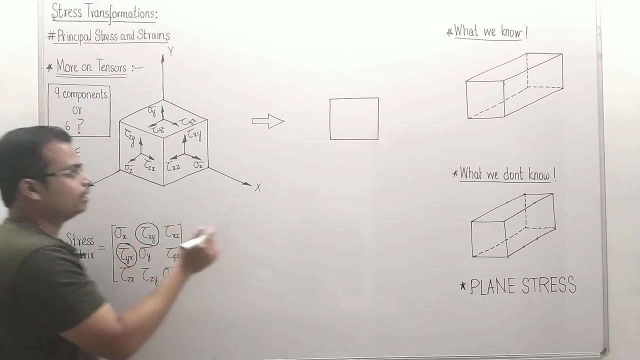 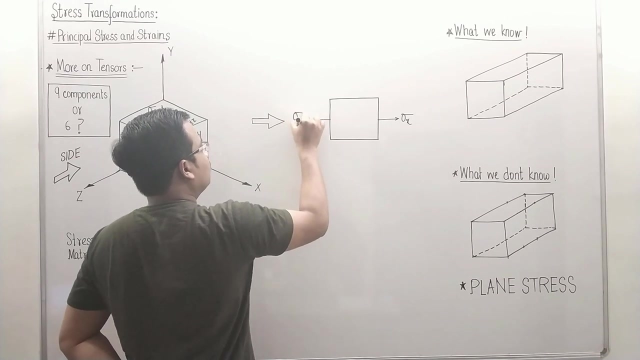 side, let's say we are having the side view. then the arrangement will be something of this sort: Here we go. Well, the face is going to look something like this, isn't it? There is going to be sigma x, sigma x, there is going to be sigma y and sigma y. So let me just make them this over: here is sigma x And that's sigma x, That's sigma y, And this also is. 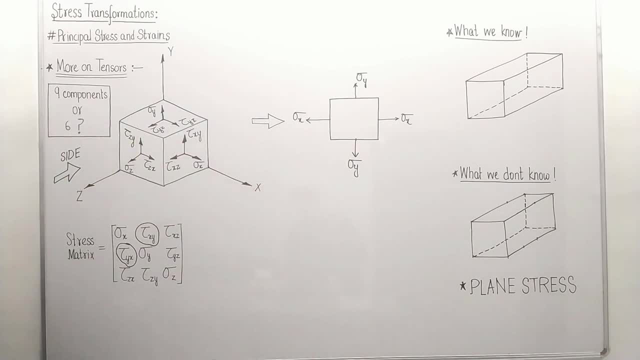 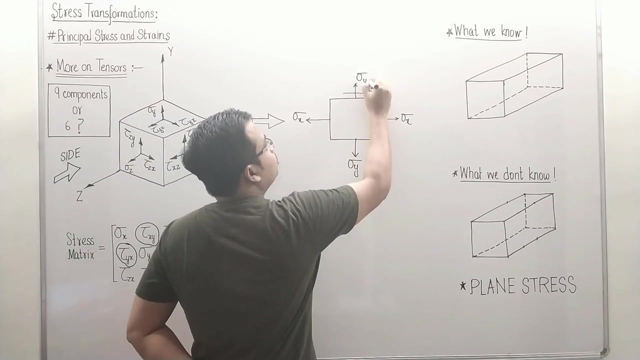 sigma y Done. What about the shear stresses? If you watch along this surface? okay, not this direction, but in along this direction, this is tau y x. So this over here is tau y x, Just like there is tau y x along this direction. in the bottom surface also, there is going to be tau y x, but in the opposite direction. This is tau y x by u. This is again tau. 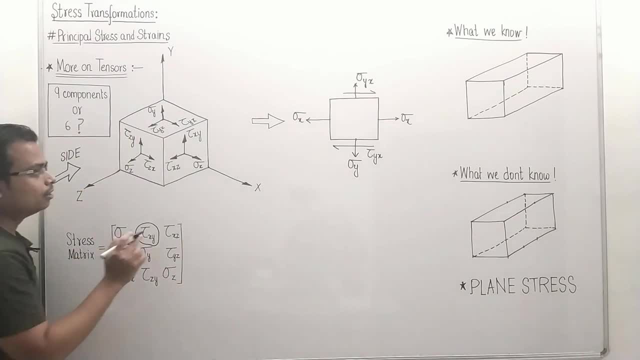 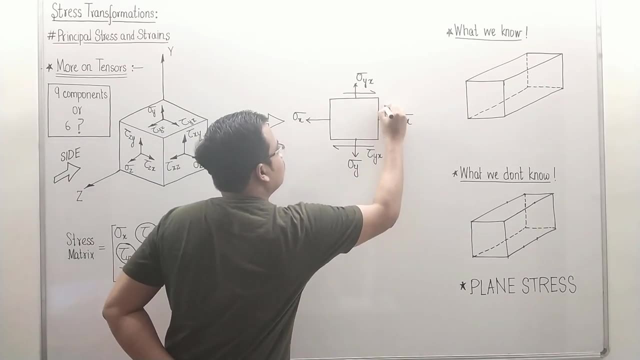 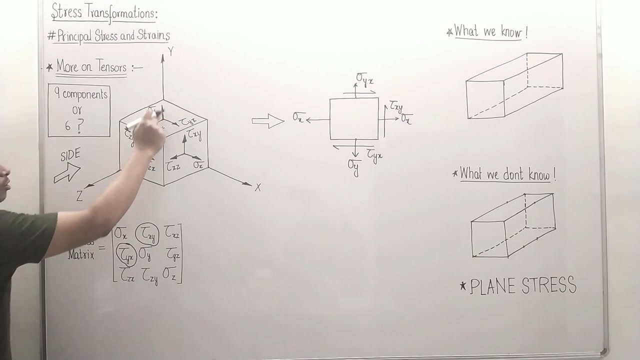 y x. Again, take a careful look. This is tau x y in the upper direction, This right hand side face. That means this one. This over here is tau x y And somewhere along this face over to the side. 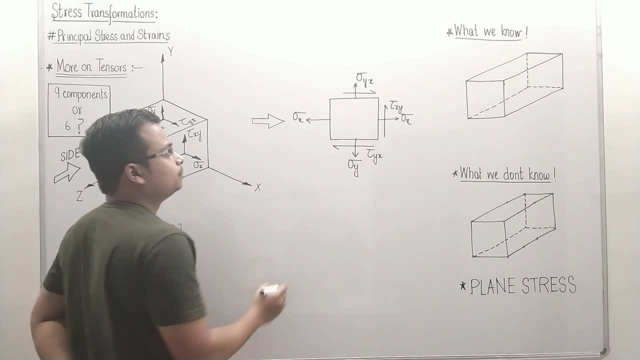 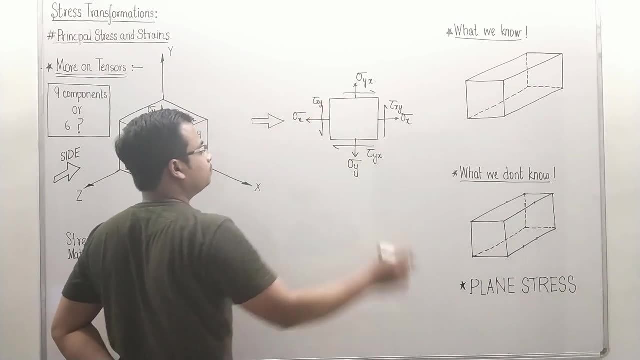 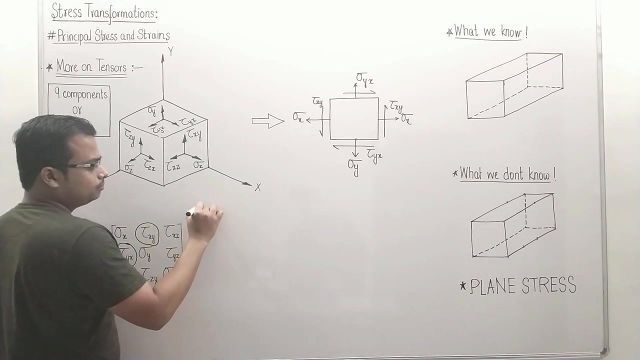 we will have this tau x y in the bottom direction. This way, This way, Tau x y, Isn't it? Now, you know, this entire system has attained a state of equilibrium And whenever any body, any particle is, 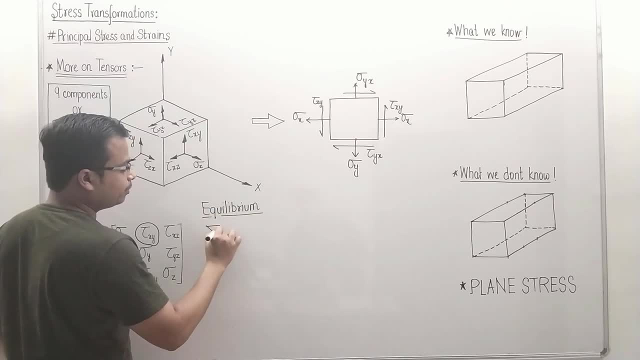 in a state of equilibrium, we always have these two equations working with us. Summation of all the forces along x, y or z direction will be equal to 0.. And also summation of rotation, let's say torque, let's say moment. 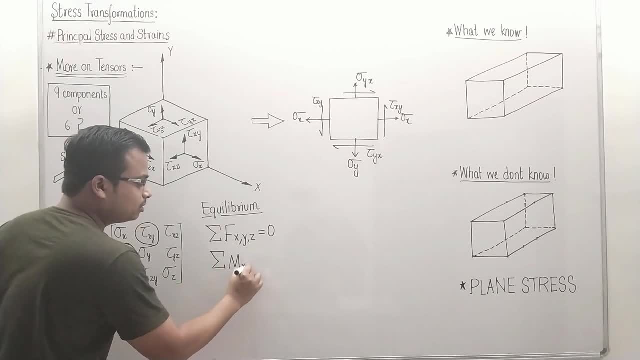 of all the forces with respect to x axis, y axis or with respect to z axis is also going to be equal to 0. So we are viewing it from here. In that case, the rotation or the moment about the z axis will be equal to 0. So here it is. 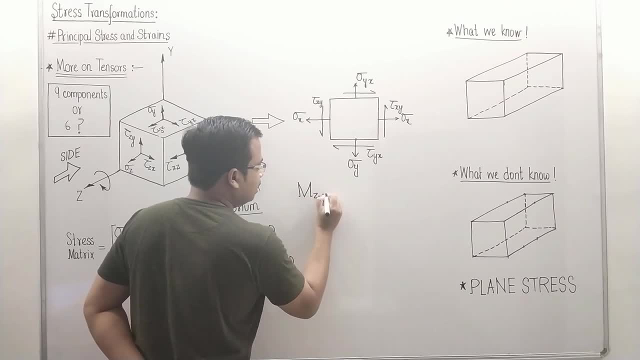 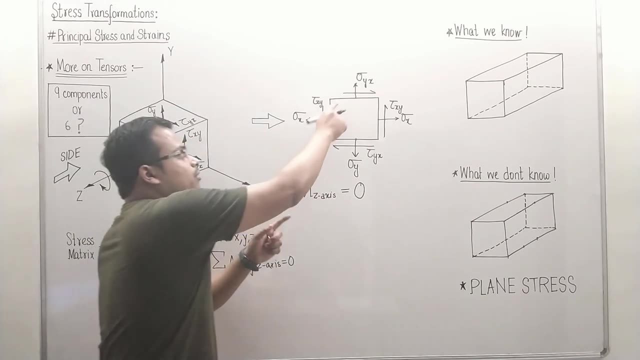 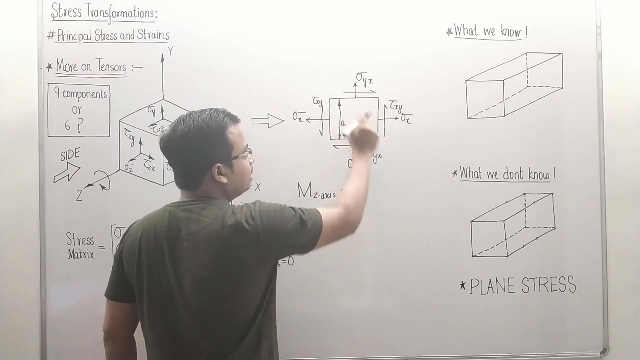 Moment about the z axis. z axis is equal to 0.. Isn't it Okay? So these are the two forces separated by a distance. Let's say, this is the distance a, And this over here is a square, So that's a. 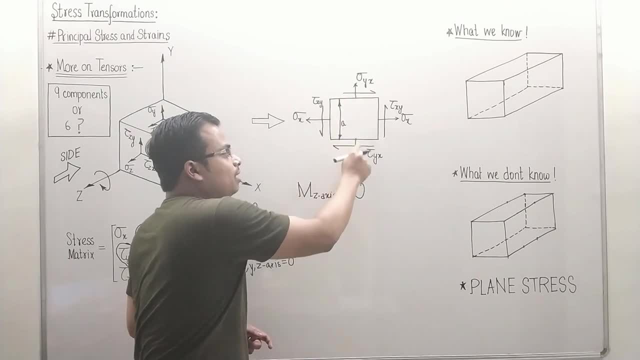 and that's a Two forces which are parallel to each other. Now these can be converted into forces also. Let's say, at the top the area is a. In that case, this force over here, this stress, can be changed to a force and I can just write a over here. 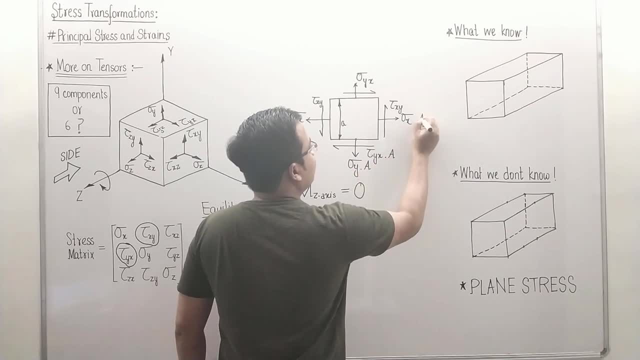 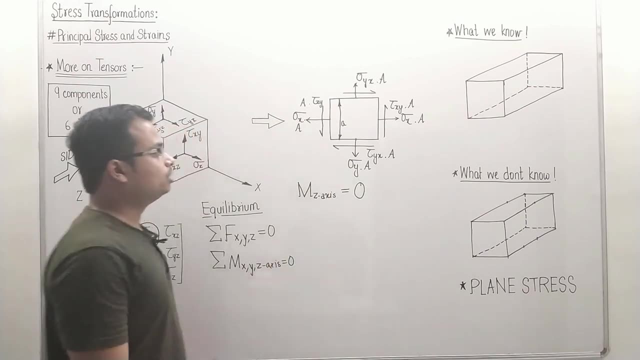 If I just multiply a over here, this will become a force, All of them. If I just multiply them with a, they would become force. Isn't it So? these are all the force acting on this element, Isn't it So? two forces. 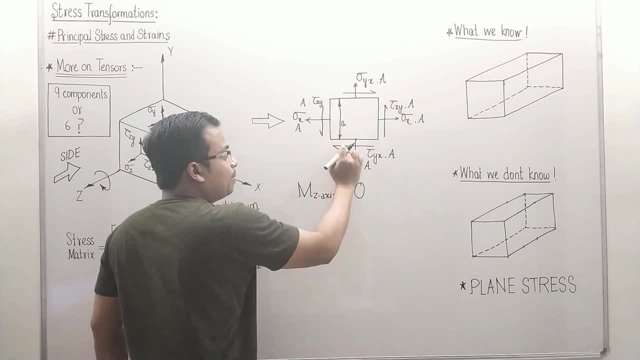 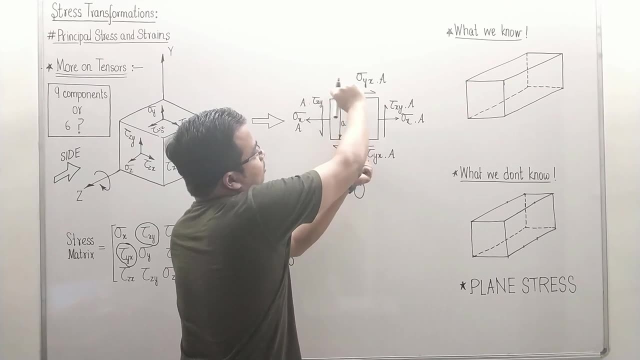 separated by a distance. Two forces are parallel. separated by a distance, They form a couple. So this over here, if you watch this, what sort of a couple is this? It's a clockwise couple And for a clockwise couple you need to take the positive. 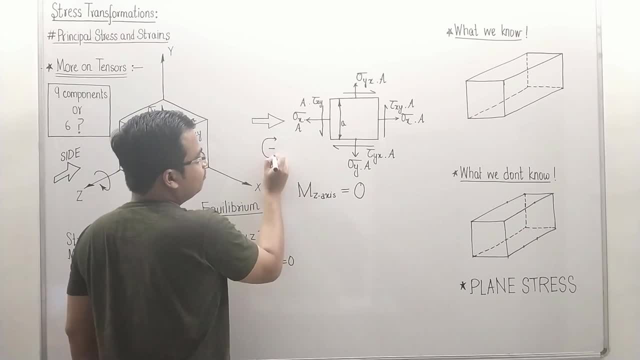 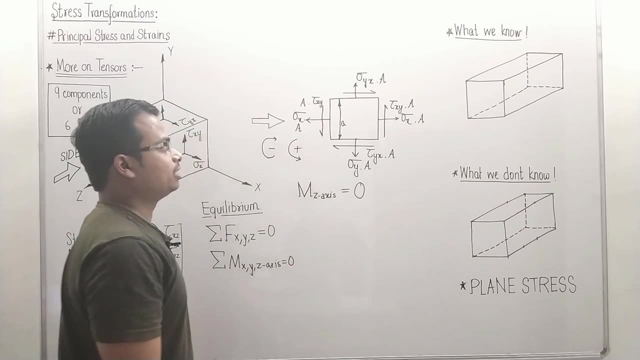 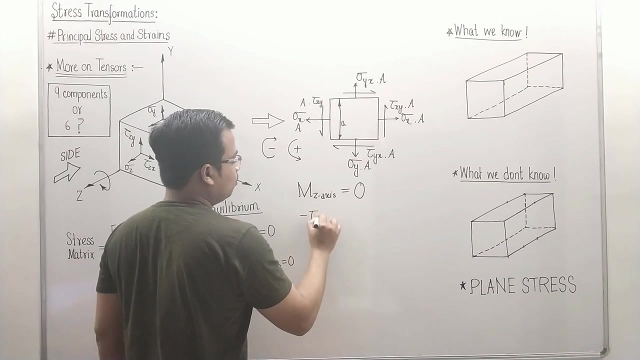 Rather negative direction or negative sign. And for an anti-clockwise couple you need to take the positive direction. So tau y x, Okay. So this is clockwise minus of tau y x, dot a, And this over here, tau x, y, If you watch. 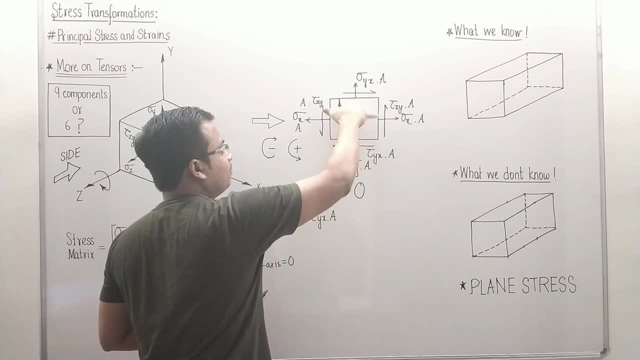 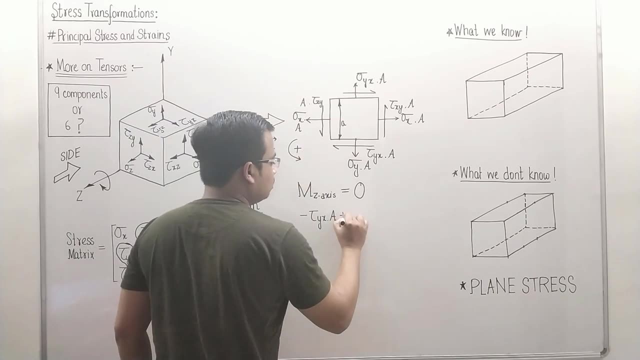 this. this is upwards and this is downwards. What sort of an effect is it producing? This is an anti-clockwise effect, And for that you need to put a positive sign. So plus this is going to be tau. What x, y, x, y, multiplied by a, and all of this is? 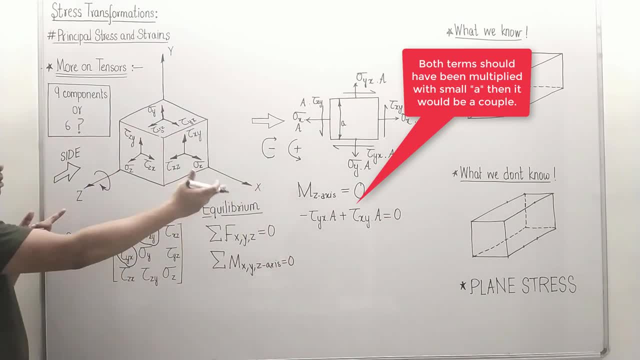 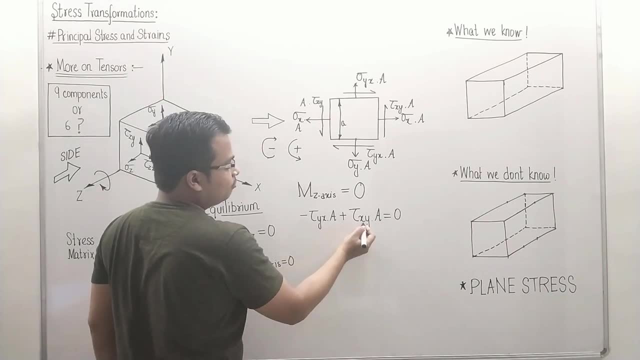 going to be equal to zero. Now, since the object is in equilibrium, you can do this stuff with respect to x axis also, with respect to y axis also. That can be done. In that case, a and a will cancel out Tau x. y will be equal to tau y x, So tau y x is. 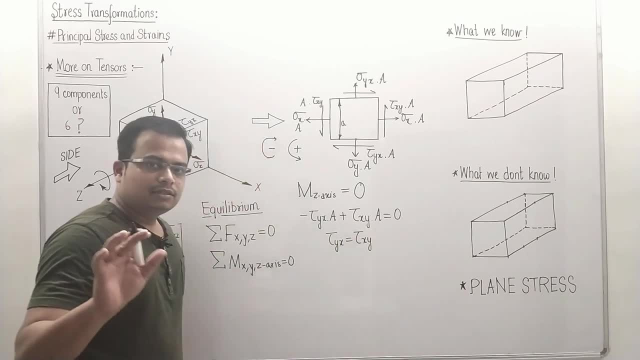 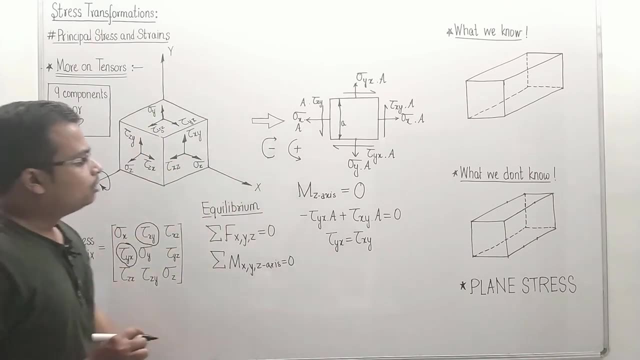 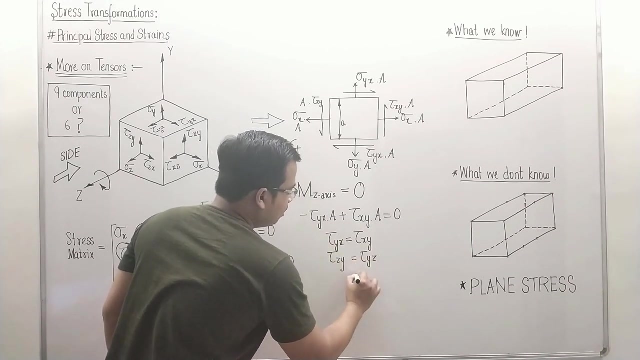 equal to tau x, y And, guys, in the same manner, if you take the moment about x axis and if you take the moment about y axis, you will realize. you will realize that tau y z will be equal to tau z y and tau z x will be equal to tau x z. So, effectively, these are the three components. 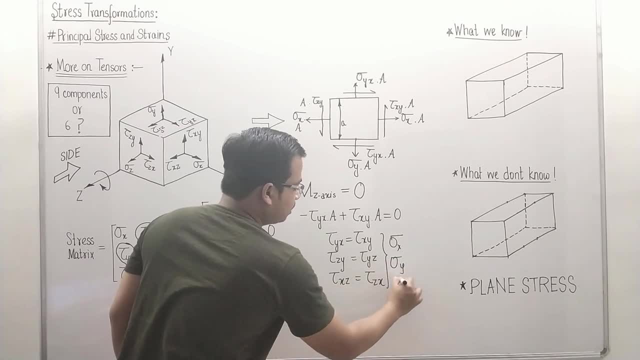 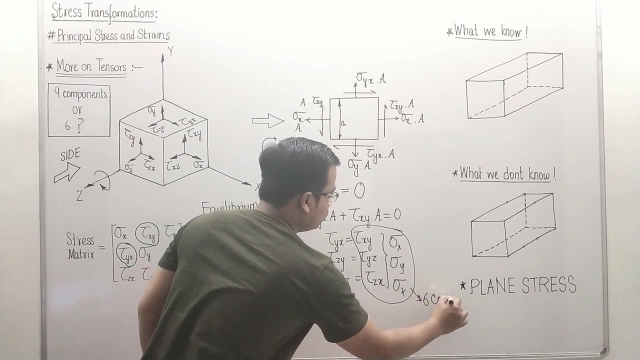 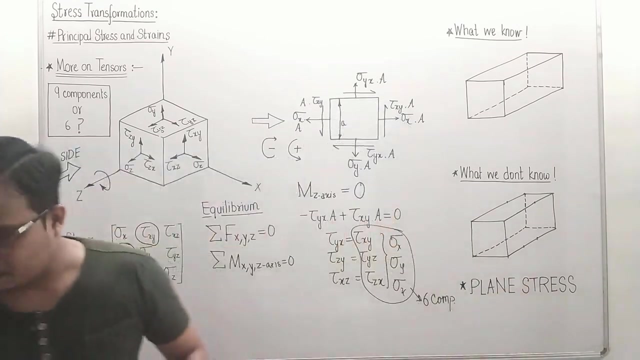 plus sigma x, plus sigma y and plus sigma z. So in totality, if you just make a count, there are effectively six components of stress acting at a point inside a rigid bond. Done Okay, so let me just wrap this and let us start the main business. Okay, Okay There. 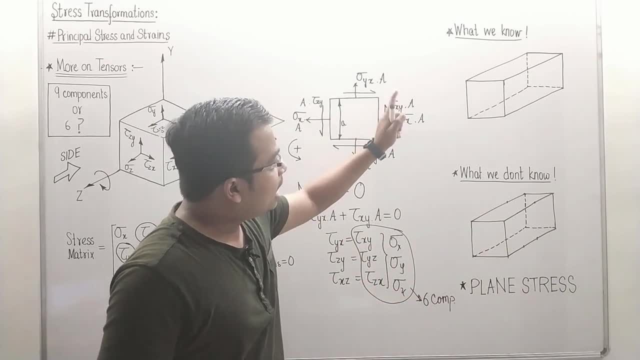 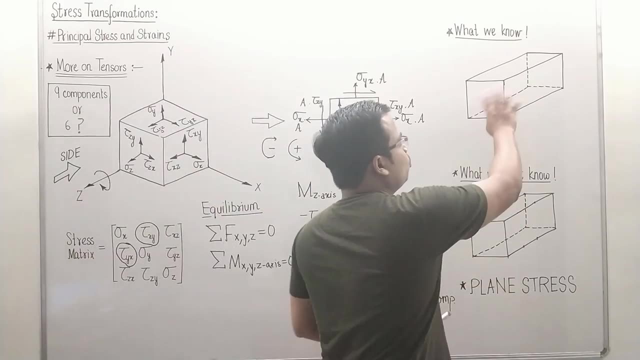 is something else which I will have to tell you: what we know and what we don't know. and what exactly is plane stress? Right, What we know. Okay, so this over here can be assumed as a cuboid. Now, let's say, this cuboid is being acted upon by a force like this. 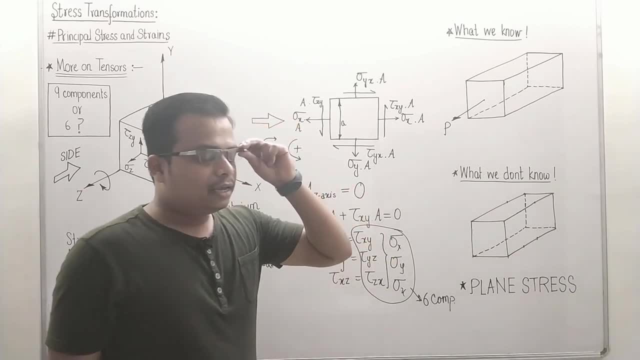 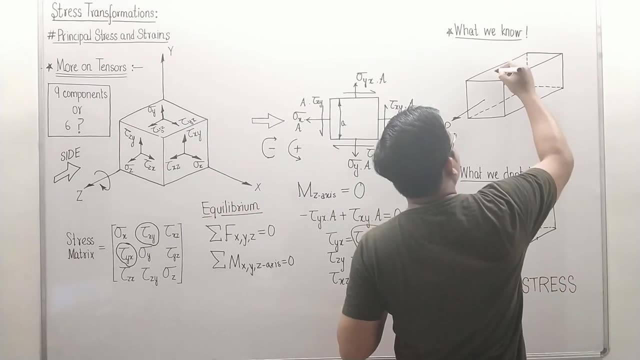 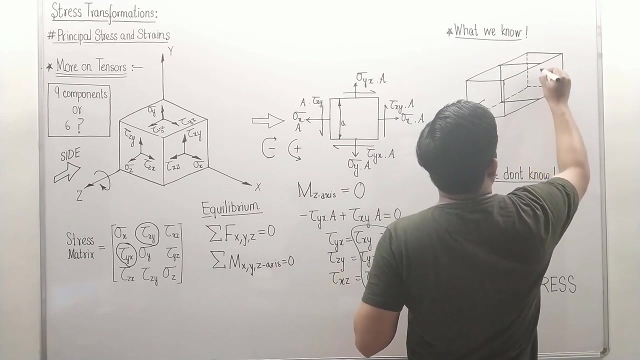 Okay, let's say that the force acting is P. Now, if I tell you that, can you tell me how much is the normal stress induced? Well, you can do that very easily. You will see that normal stress can be calculated very easily along any cross section like this: 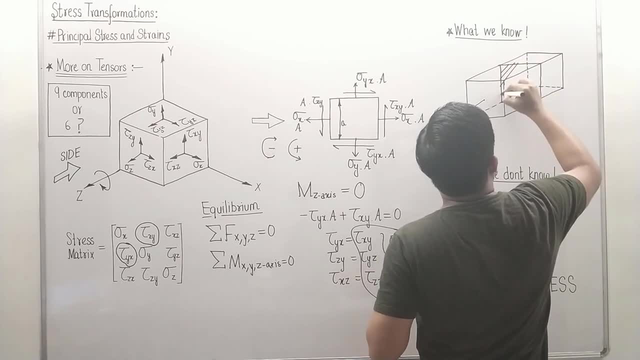 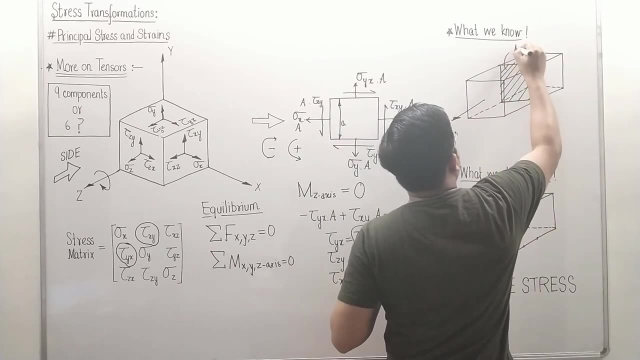 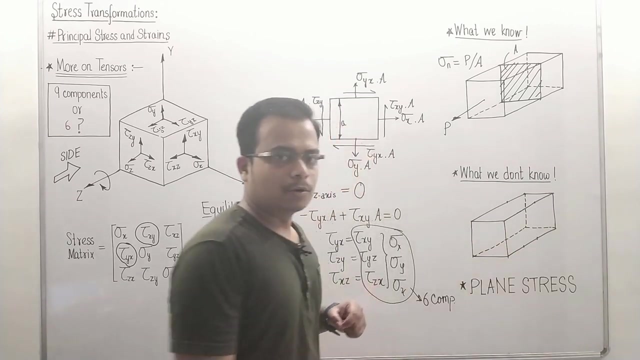 So in this cross section, in this cross section we can actually calculate the value of stress. Let's say, this area is A. In that case sigma n, or the normal stress induced, will be equal to P by A. Okay, fine. 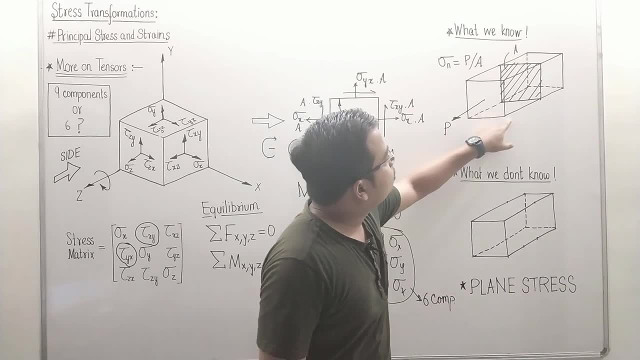 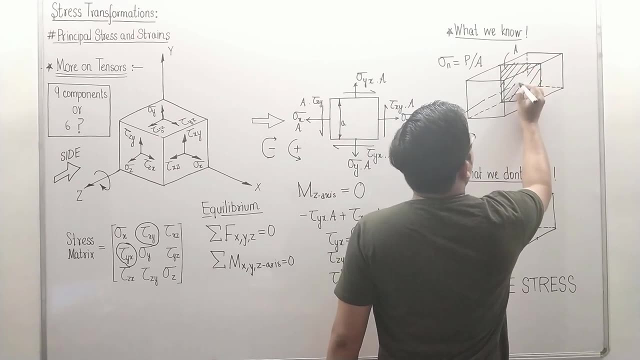 That means we know how to calculate the value of stress induced on a plane which is perpendicular to the axis. If I can just extend this over here, let me try to drop this. The angle made over here will be equal to 90 degrees. 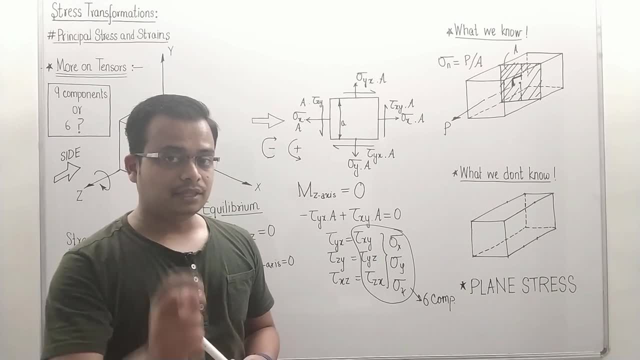 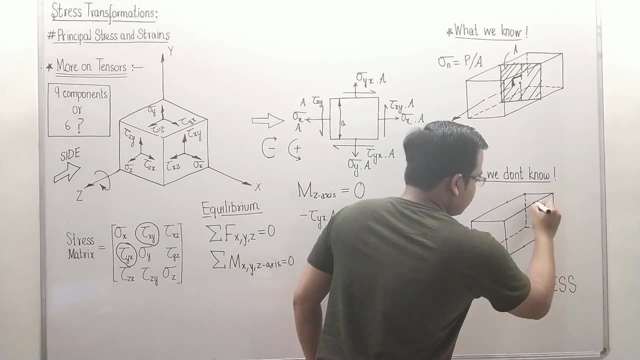 So whenever you have a plane perpendicular to the axis there, you can calculate the normal stress. But what you don't know is this: Okay, this is what you don't know. If I tell you, please go ahead and calculate the value of normal stress and also shear stress or tangential stress. 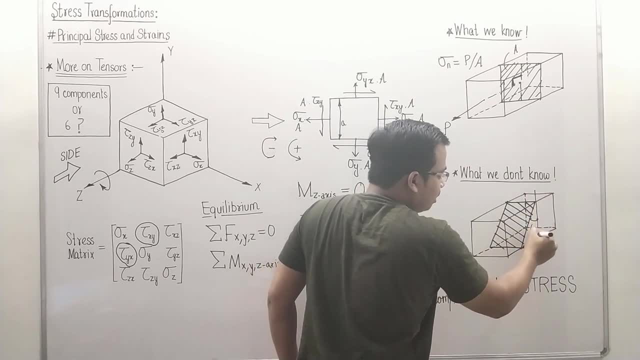 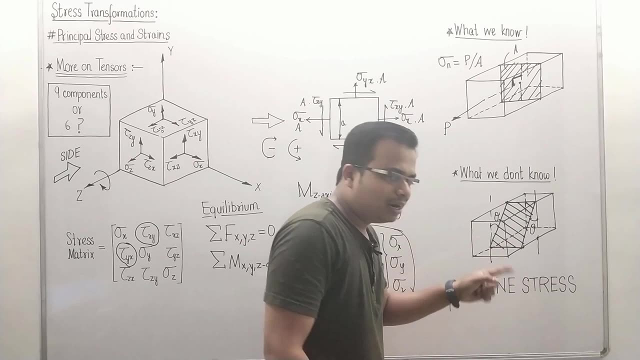 Along this Oblique plane. let's say, this is making an angle theta with the vertical. here also It is making an angle theta with the vertical. Can you tell me how much is the maximum normal stress? Or let's say in general, how much is the normal stress at an angle theta on this oblique plane? 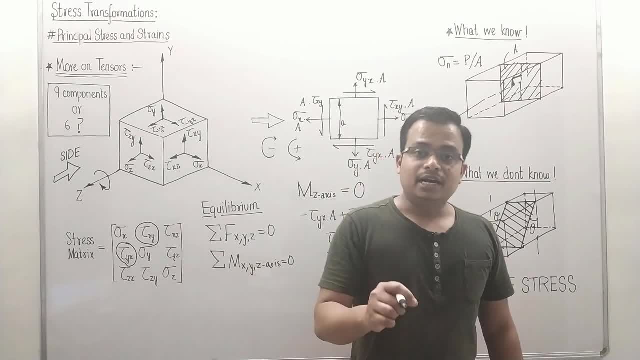 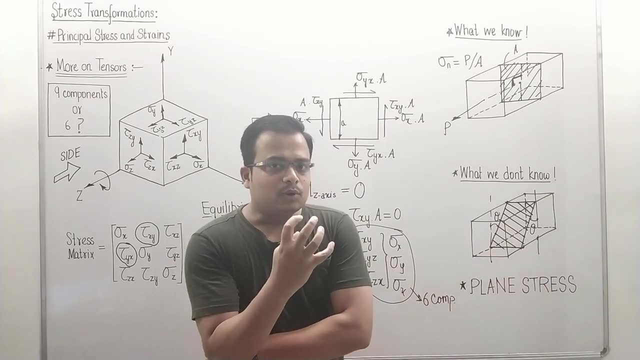 Can we do that? Well, we can definitely do that, But at the end of the video I'll try to explain you all of this stuff and how exactly you can calculate the value of sigma n and sigma t. That is normal stress. 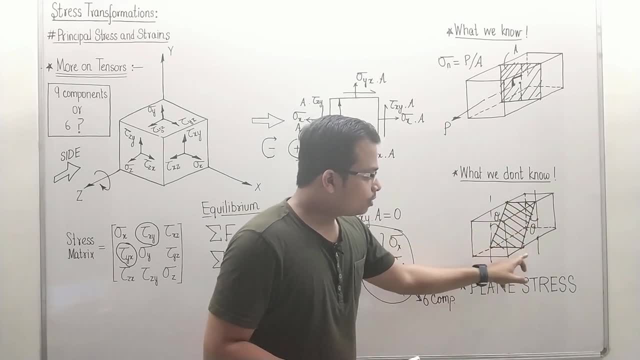 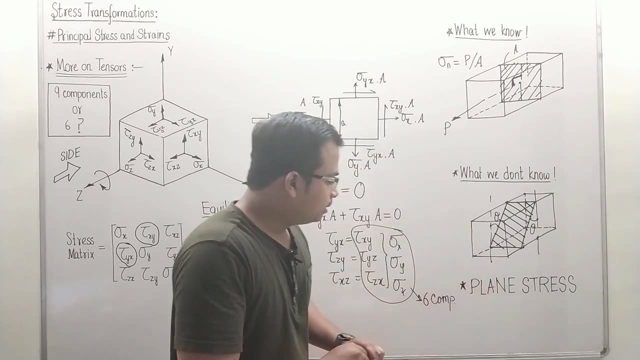 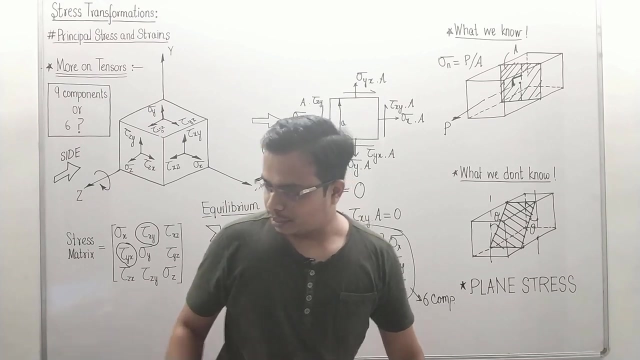 And tangential stress on a plane which sort of is inclined at an angle theta with the vertical. So all of this and much more coming up in today's session, But before that, let us have a discussion on plane stress. Okay, So let's get back on track. 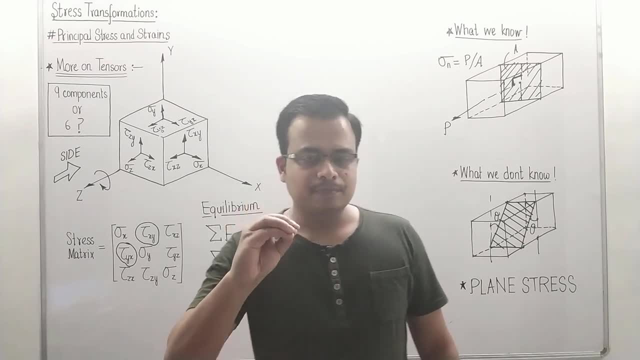 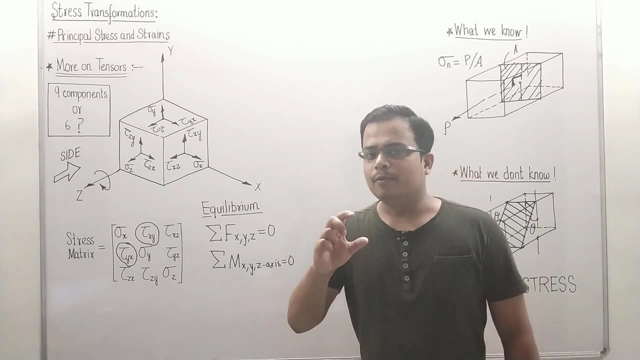 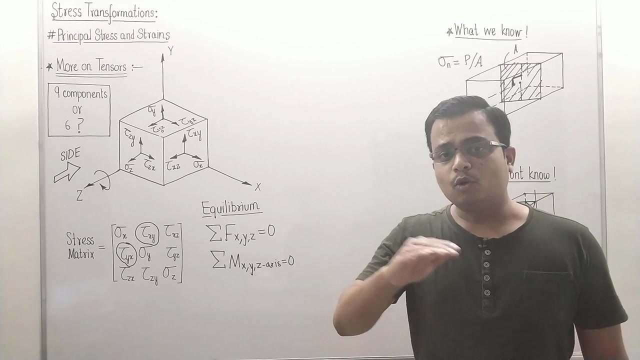 And we now know very well that there are as many as six distinct stress components acting at a point inside a rigid body. This state of stress, however, is not very often encountered in engineering applications or engineering practice. Instead, the loadings are coplanar. 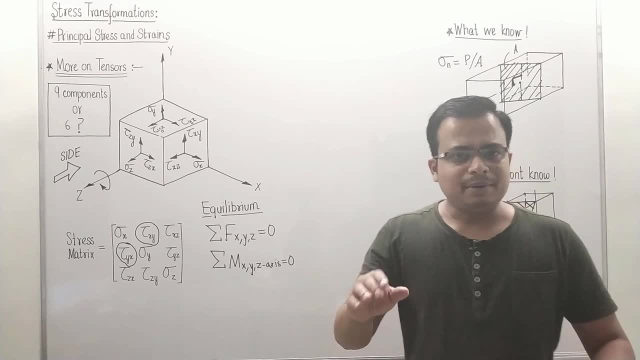 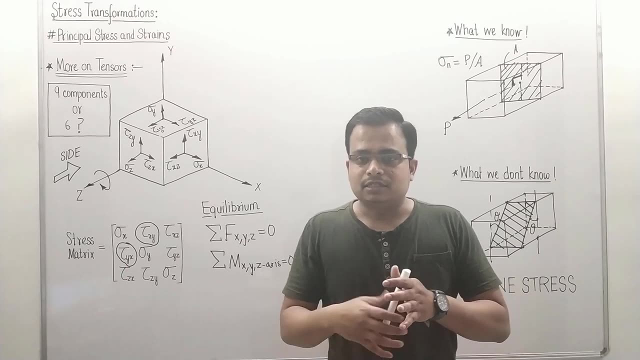 That means they produce stresses which can be analyzed on a single plane, And when this is the case, we'll say that the member or the material is subjected to plane stress. Let me just explain all of that with the help of a beautiful example. 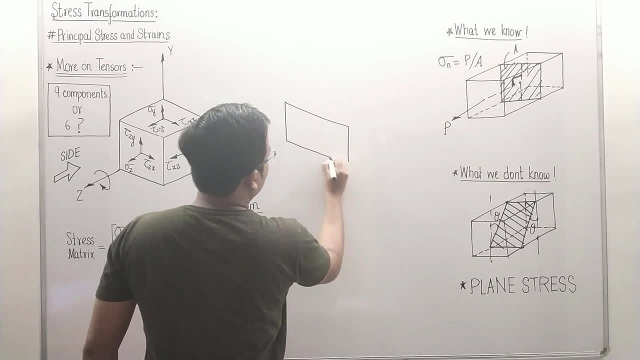 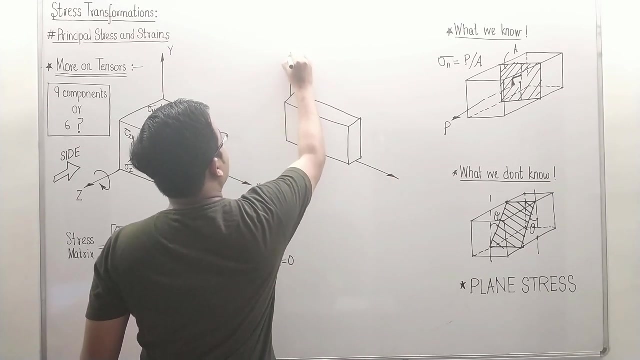 It's something like this: Let's say, we've got a Material like this. Okay, Yeah, like this. So these are the three directions. This is, let's say, x And this, right here, is the y direction. 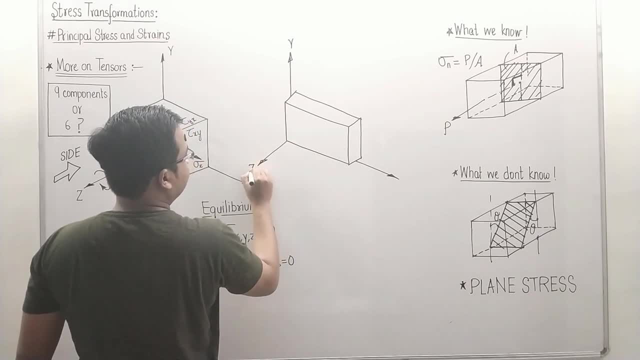 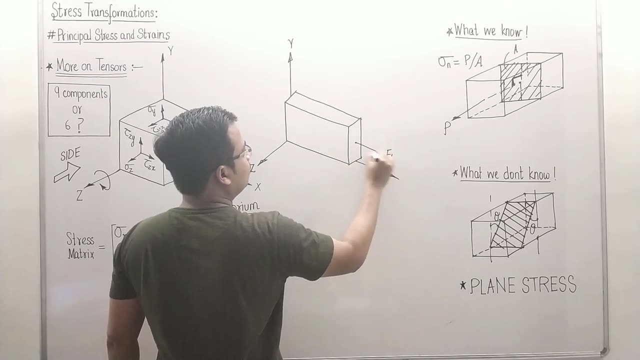 And this over here. well, let's say this is z. Now there are a bunch of forces acting. Okay, This, let's say, is f1.. Okay, There is a force over here. also, Let's say this is f2.. 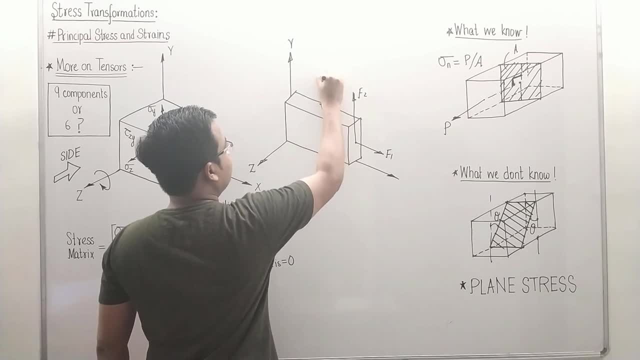 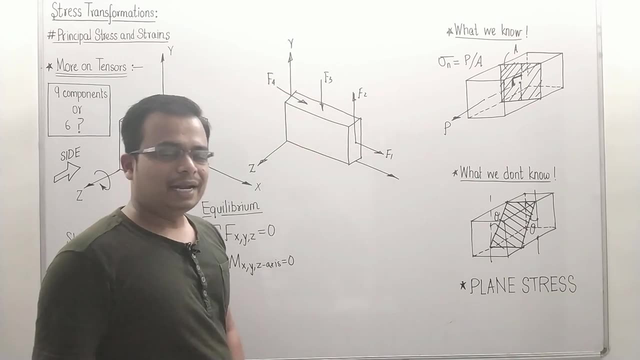 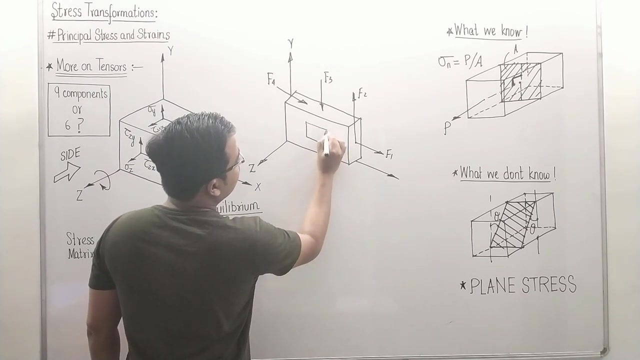 There is a force Here. This is, let's say, f3.. And then there is a force here, Let's say f4.. Now, because of all these forces, a net force is going to act Right Now, if you consider a very small element, very small element like this, because of all these forces, right, 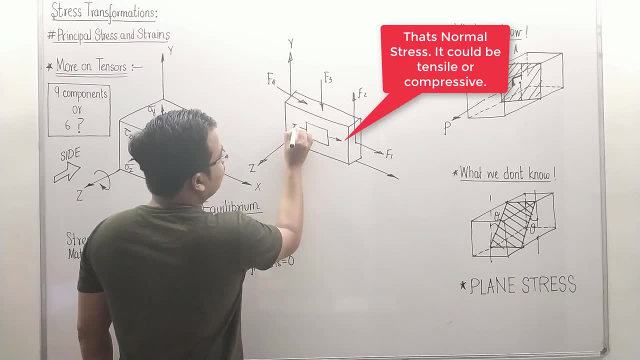 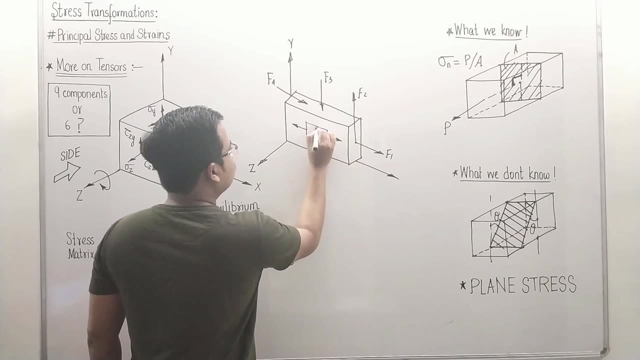 So there is going to be a tangential stress along this x direction. This is going to be sigma x, Isn't it? Let me just? Let me just put the arrows. first of all, There is going to be a stress in the y direction also. 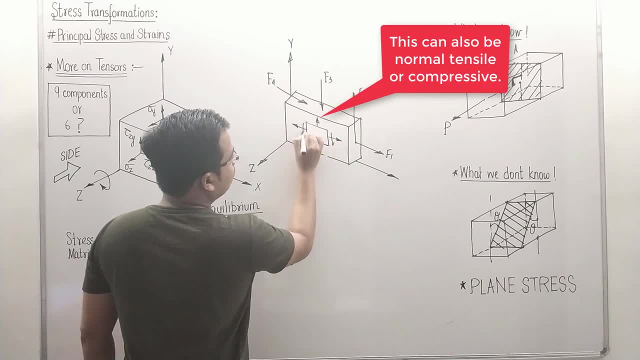 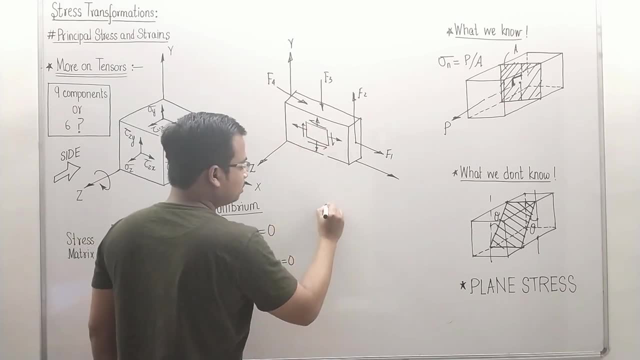 This way, And there are going to be shear stresses This way, This way And this. over here is the complementary shear stress. If I were to make this in a proper sense, it would be something like this: That's the element. 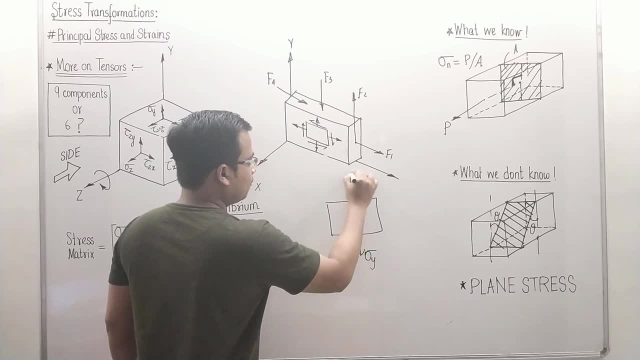 This is going to be sigma y, Sigma y. This is sigma x, Sigma x. Then we have this: This is 0. That's here. We have a formula: andotomizor. Now again we have a formula: is at O, there is going to be a shear and nanofaradion. 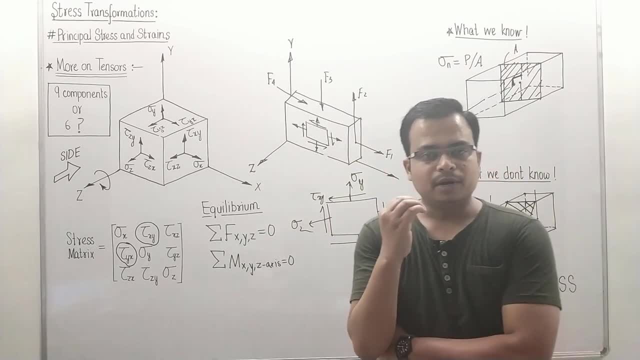 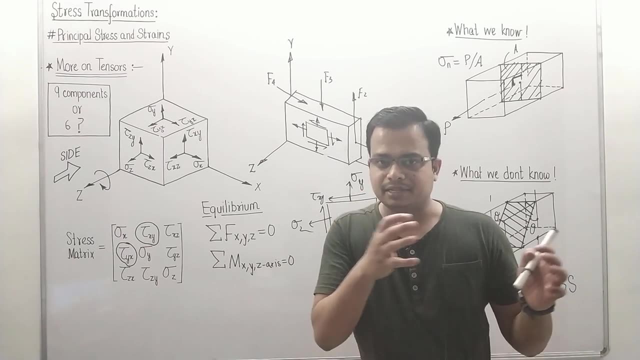 but we are going to take 0.. So this one is going to be O, this one is going to be sigma y. Do you ready? So these are correspondingители for the noise, because the laser has a shear, and they aremetric сейчас along the line. 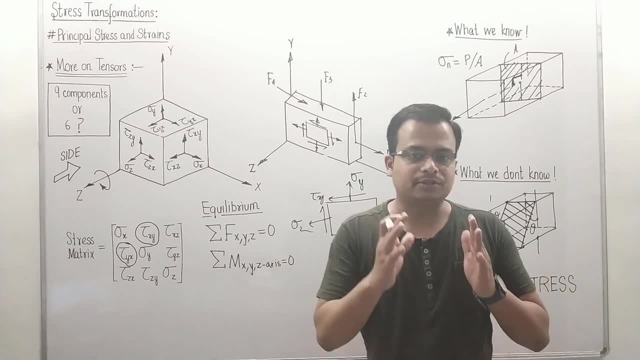 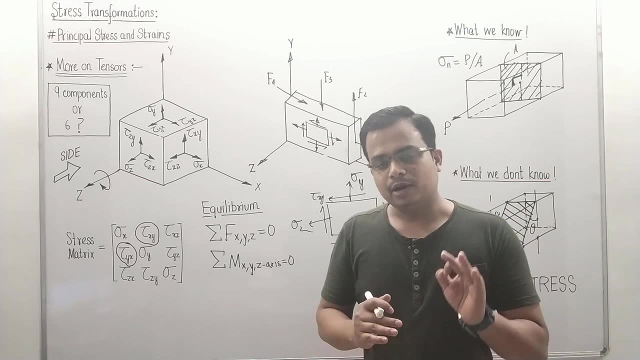 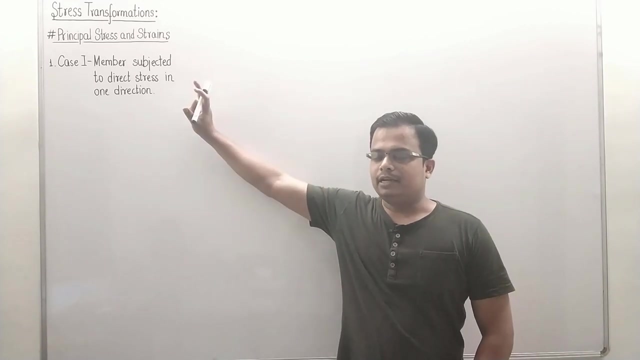 And that's it, Isn't it? two directly mutually perpendicular stresses plus shear stress. So these are the four cases that we are going to take up, But in today's video I'll only talk about case one. So let's start with case one. Here we go. So now let us start with case one, that is, when a member 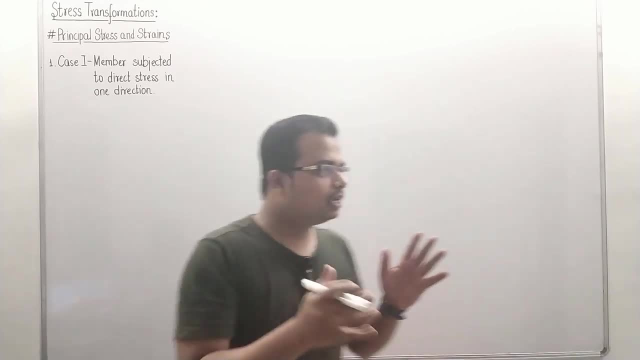 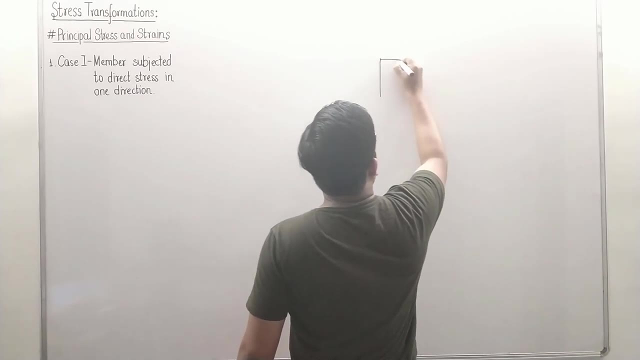 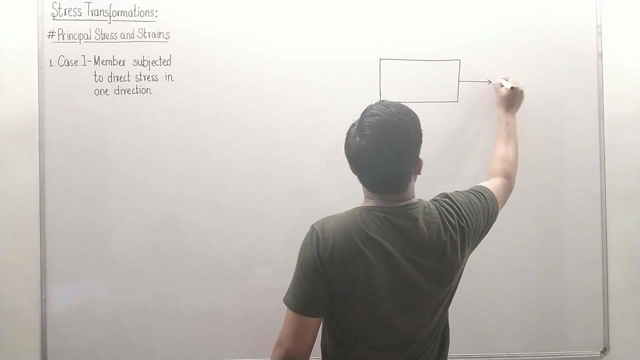 is subjected to direct stress only in one direction. let's say we are talking only about the x direction. So here is the analysis. So first of all let us try to make a member, and if we rather make a bigger figure, there is only one stress acting, let's say in the 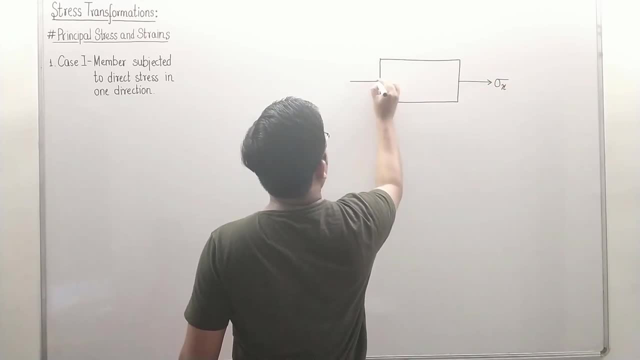 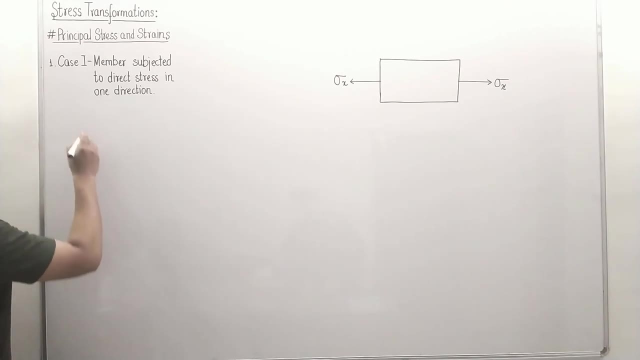 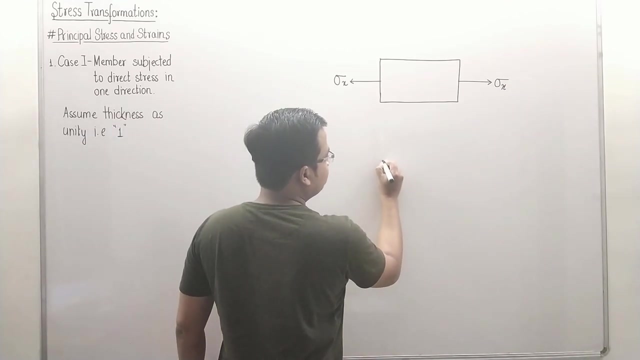 x direction. let me call that sigma x. Okay, that is sigma s. By the way, the one assumption which I'm going to take is that thickness assume thickness as unity. So we actually the arrangement is something like this: if I try to make this in 3d, it would be: 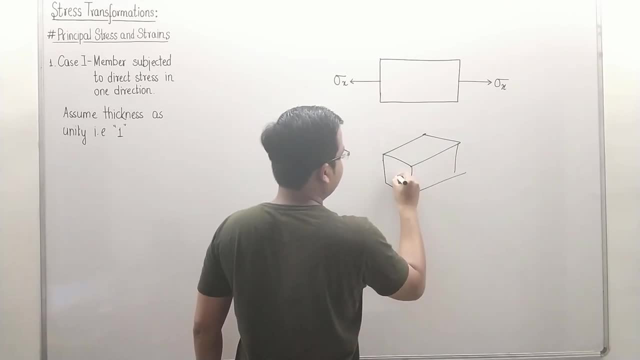 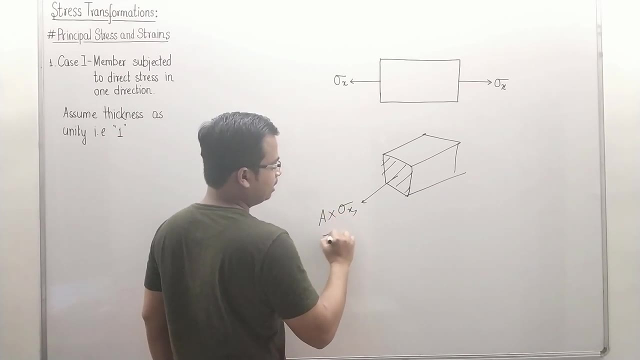 something like this: Yeah right, So this is sigma x, So this is the area. So if you multiply sigma x with area, you'll get the value of load applied in this direction, that is, p x. So let me just write. 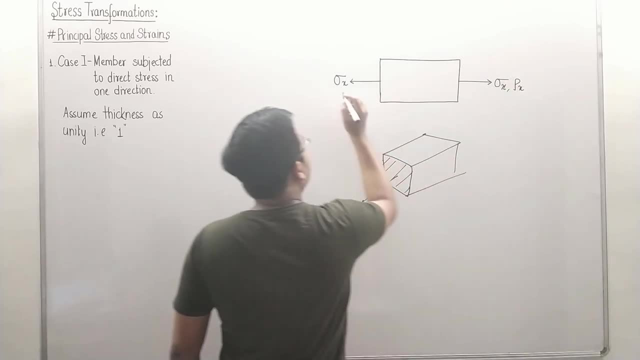 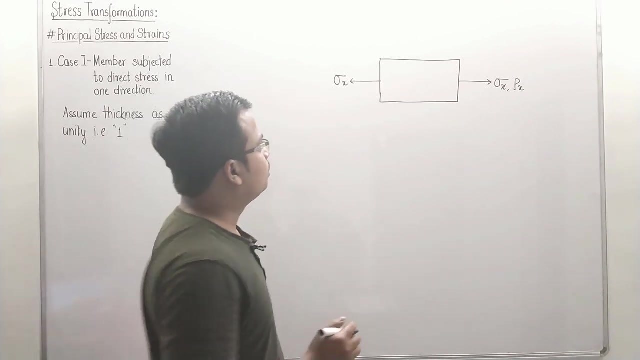 p x also over here. try to have a better picture, Okay, just over there, not to write here. Okay, So this is what we've got: a member subjected to an actual tensile stress, And what we wish to do is to find the state of stress along this oblique plane. This is what we wish to find, Okay. 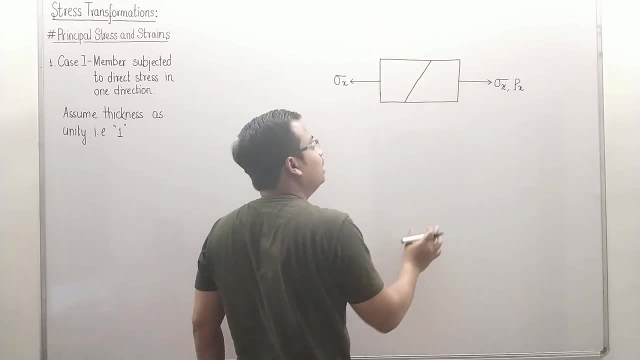 we wish to find the normal stress along this plane, normal stress along this plane, and we wish to find the tangential stress along this plane. Let's say that this, this is represented by Pq, And let's just say: okay, the angle that this makes with the vertical is theta. Over here also, the angle is going to be: 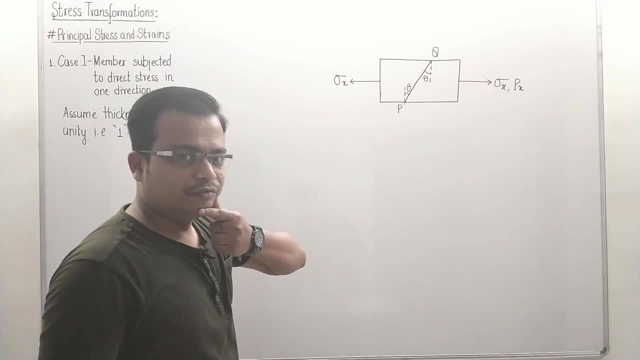 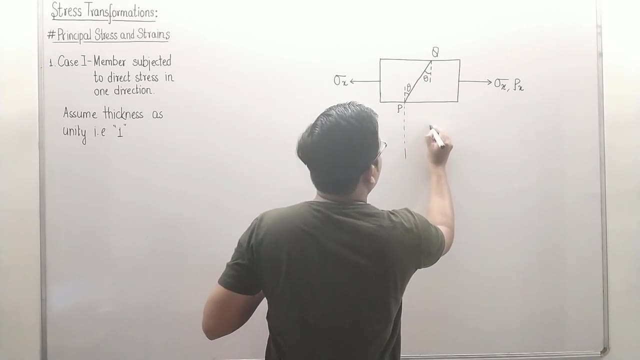 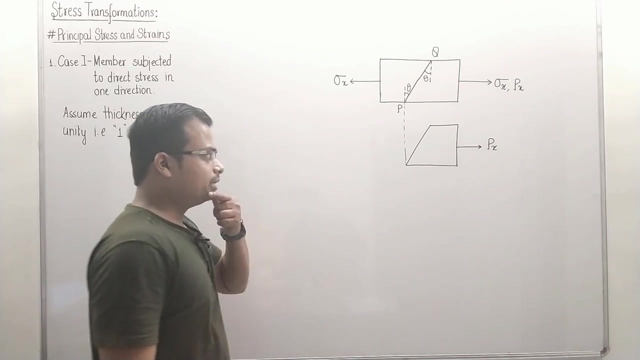 theta. How do we get this? Very interesting. Okay, let me have another figure. So let us start from here. And this way, this way and this way, The force acting, let us say, is represented by px, isn't it? So there are going to be forces acting along this plane: pq. 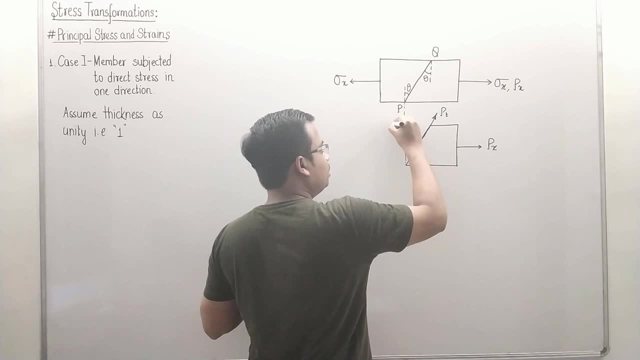 Let us call that as pt, And there is going to be a force acting in a direction normal to this pt. First of all, let me just write this pq: This over here is pn. Okay, so there is a bit of geometry. 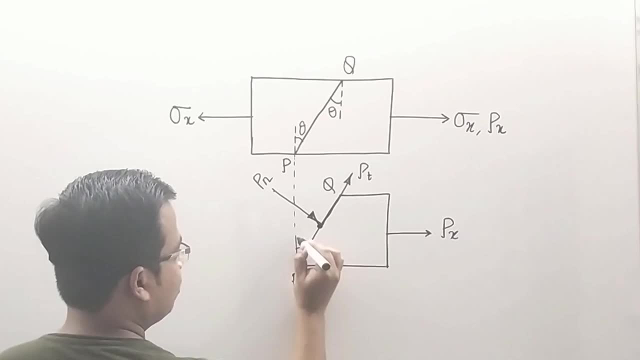 which we need to encounter right now. This angle over here, by the way, is 30. So the angle over here is going to be 90 minus theta. Sorry, not 30, but theta. So if that is the case, then the angle over here here. just try to work it out. Let me make this properly. 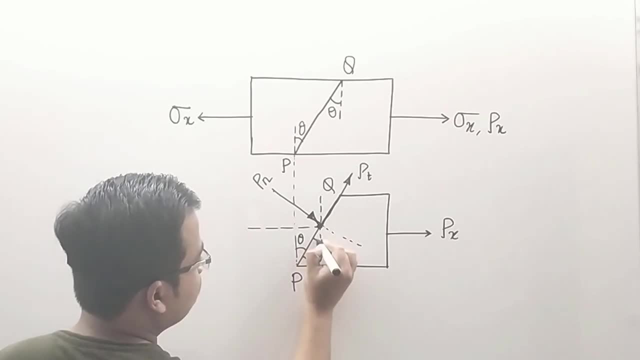 Okay, so that is 90 minus theta. This is going to be how much? If this is 90 minus theta, this has got to be theta. Okay, that is it. That is quite obvious. If this is theta, right, then this also is going to be theta. 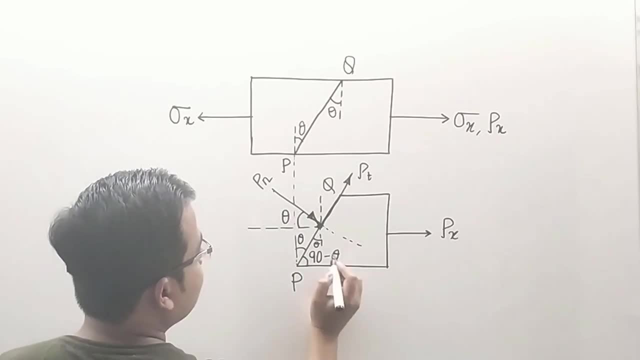 That is for sure. Just try to work it out. This is fairly simple. If this is theta, this again has got to be 90 minus theta, And if this is 90 minus theta, this is theta. If this is theta, between these two lines: if this is theta, then between these: 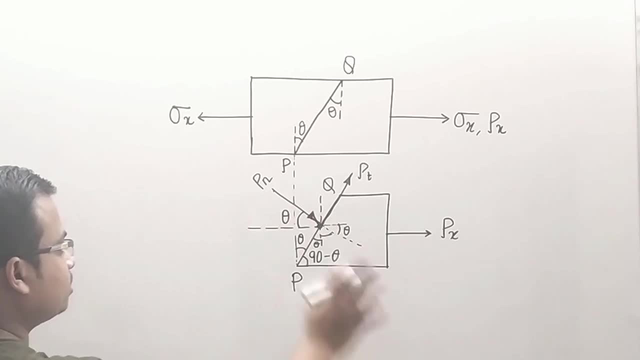 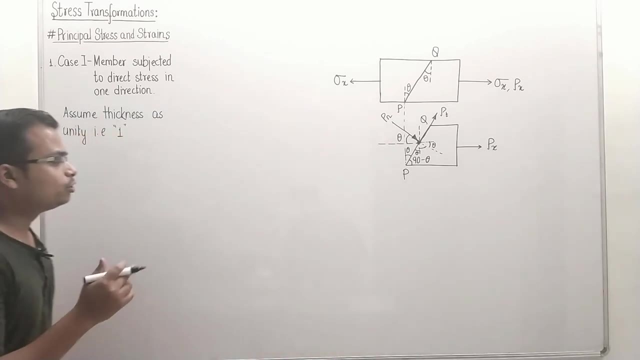 two lines. these two are vertically opposite angles. That is theta and that is theta Done. That means what we can do is here we go. Let me just start calculating. what we wish to find is normal stress. normal stress P N. 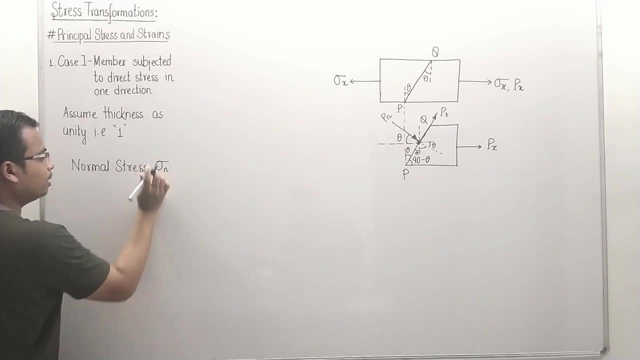 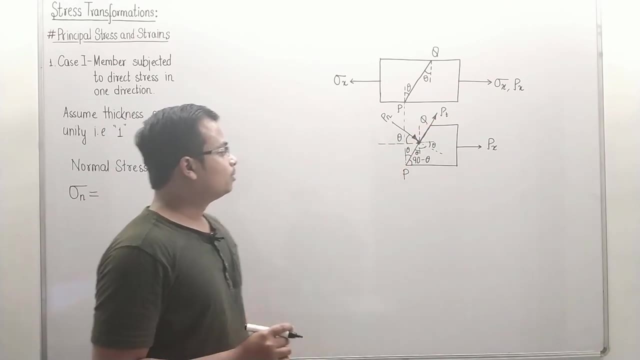 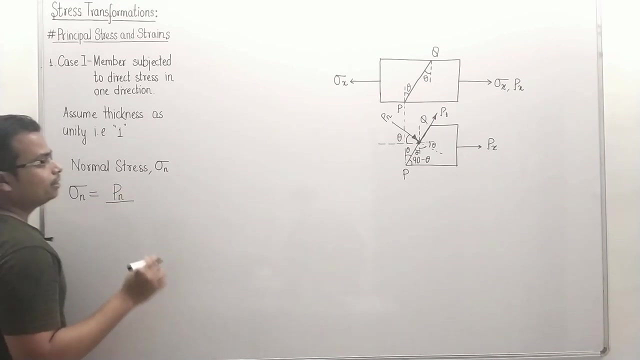 not P? N but sigma N. Okay, so, guys, here it is normal stress where Along this plane peak, So that is going to be equal to the load acting normally. that is P? N divided by area of this. 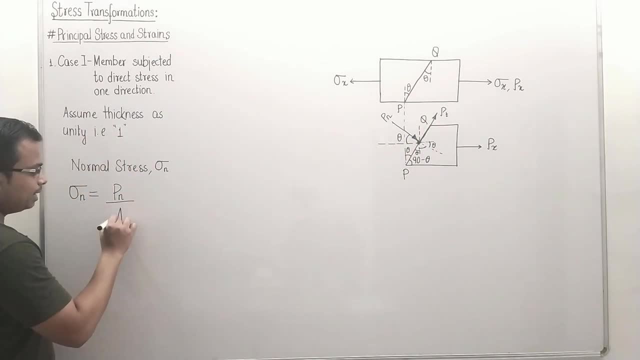 oblique plane Area of this plane, let's say, is represented by area PQ. Now, how can this be worked out? So PN can essentially be written as component of PX along PN Whole divided by that's area PQ. This is fairly easy. This is going to be fairly easy, Trust me. Okay, just keep watching. So the component. 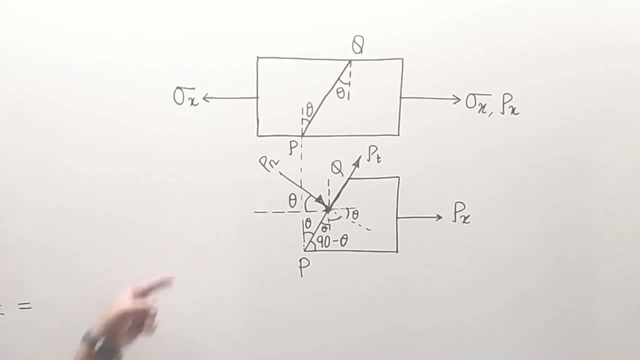 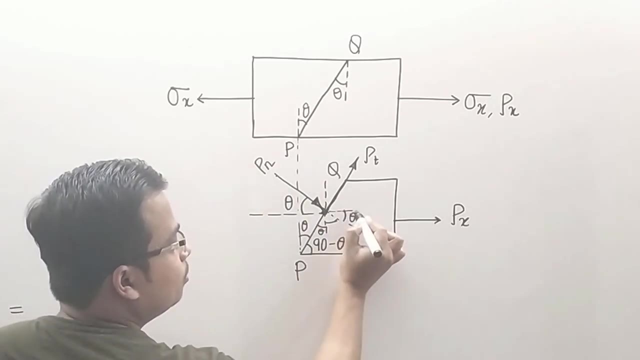 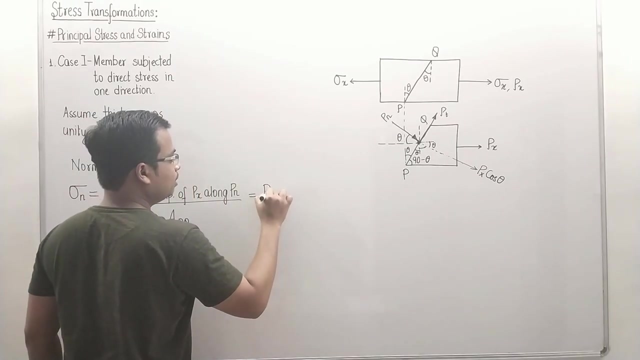 of PX along PN. Here it is. What is this PX So we want? we want the component of this PX along PN. So if this over here is PX, This is theta, Then this has got to be, this direction has got to be: PX cos theta. Okay, it's very simple. This is going to be PX cos theta divided by What is. 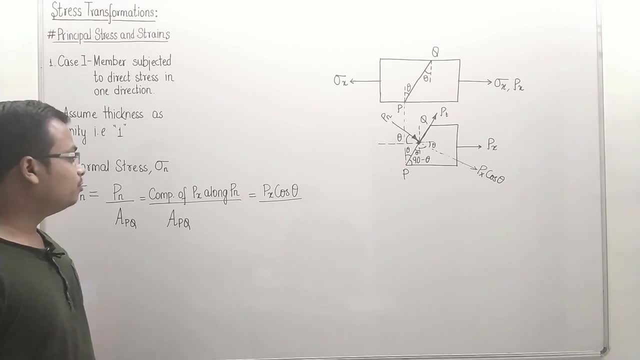 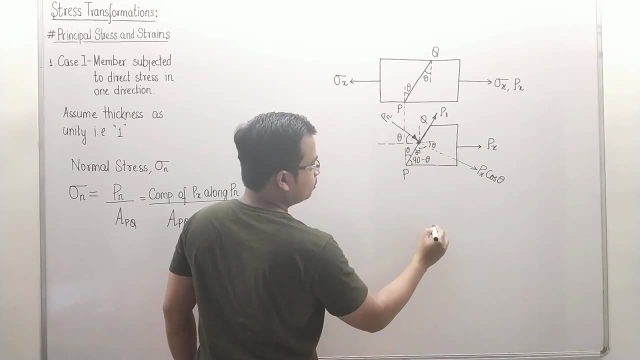 this area, P, PQ. This sounds a bit confusing. Well, it's not that confusing. Let's say, we are considering this triangle, Okay, this triangle. So so it's, it's something like this, Right, Something like this: This way. So we know this area, We want to know this area. That's PQ area. Okay, Now this angle. 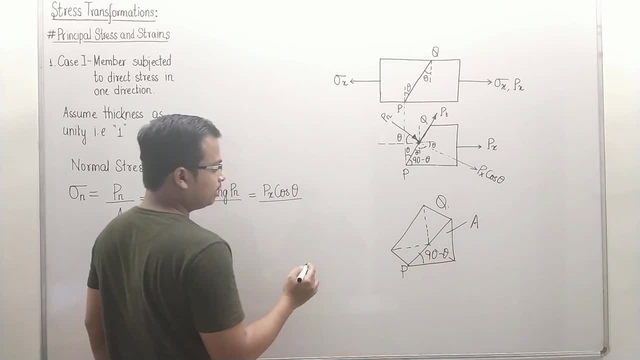 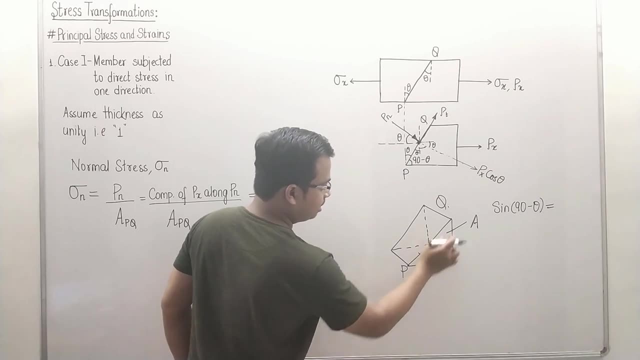 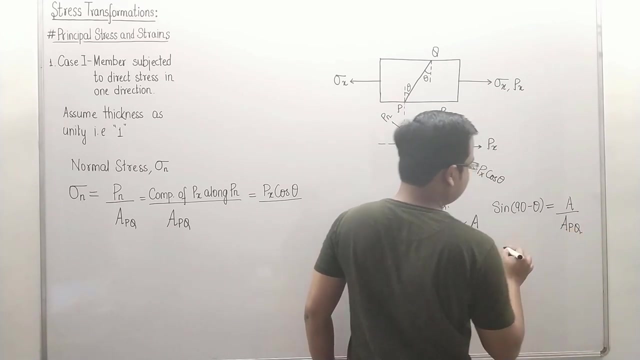 over. here is how much. This is 90 minus theta. So what you can do Is you can write: sine of 90 minus theta is equal to sine of 90 minus theta is equal to A divided by this area, A PQ, A divided by A of PQ. In that sense, you will have this. This is cos theta, by the way. 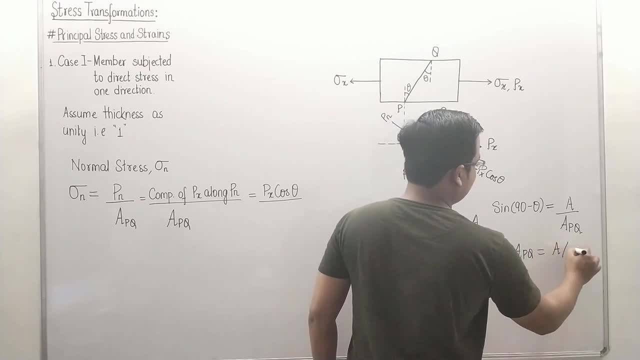 And A PQ will work out as A over cos theta. Now, this is a known fact. Let me just write this somewhere. Okay, Let me just write it over here. So the oblique plane is going to work out as A over cos theta, And this is something which we'll be using in the upcoming cases also. 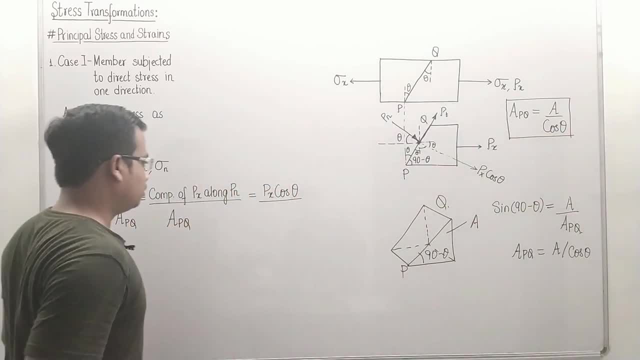 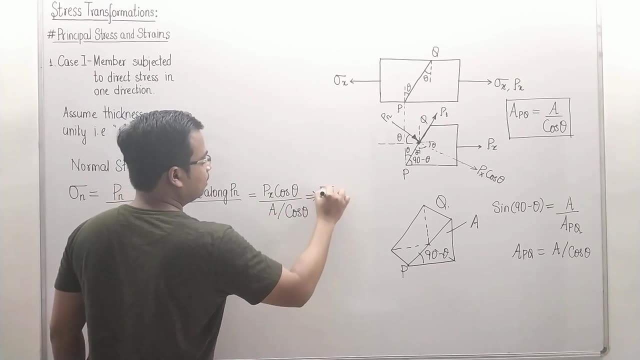 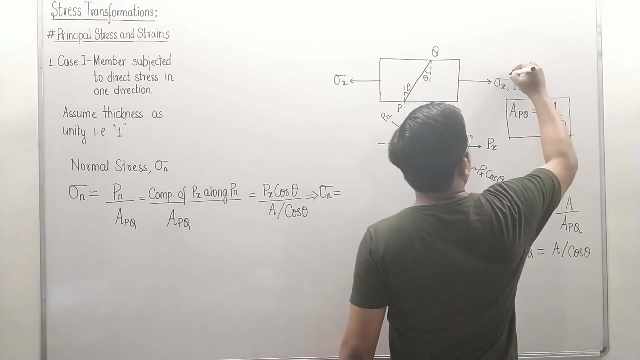 So better to memorize this. Okay, Here we go. So this is going to be how much A over cos theta, And finally you have the result. It implies that sigma n, Sigma n, will be equal to what Sigma n will be equal to. PX over A, PX over A. Here it is. If you try to relate these two, 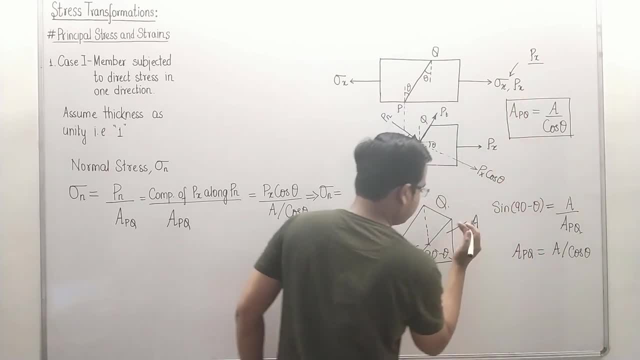 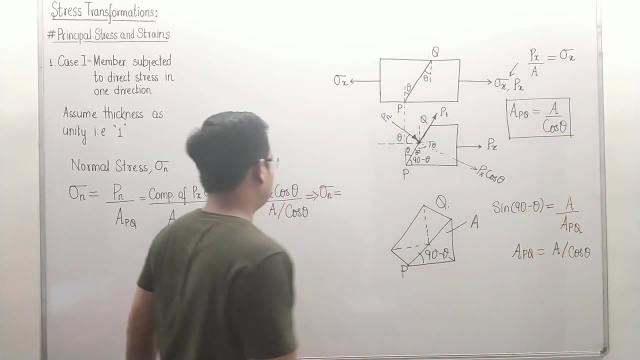 PX over this area. PX over this area, area, this area. okay, this area will be equal to sigma x, by the way, So sigma n finally works out as sigma x: times of cos. theta shifts to the numerator and this is going to be cos. 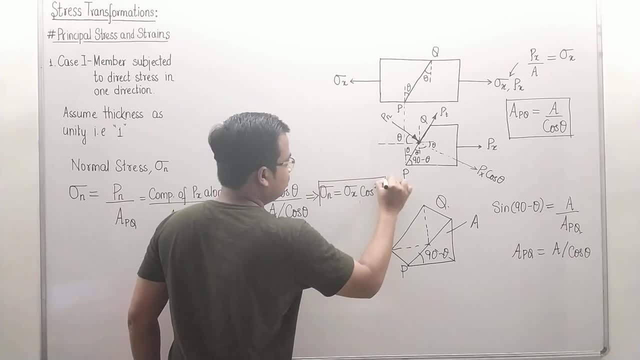 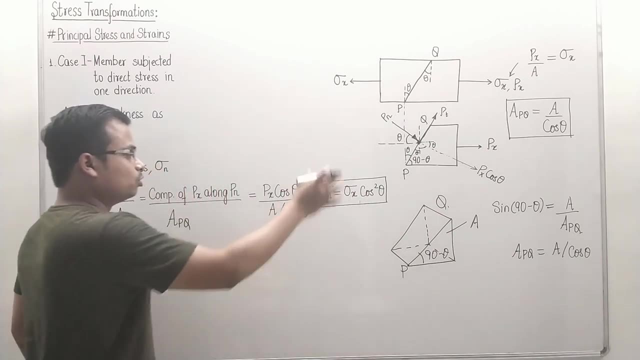 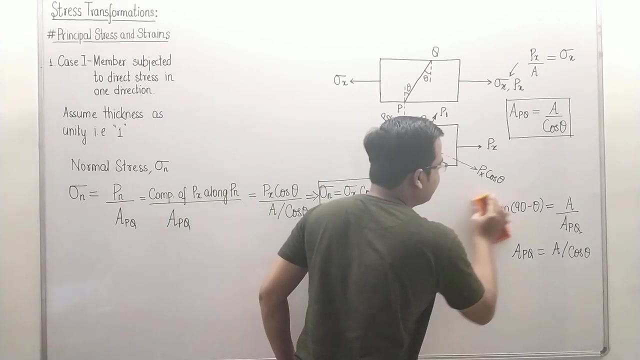 square theta. So this is the first result that we have got Normal stress onto this oblique plane. onto this oblique plane will work out as sigma x, cos square theta. And there are, just to note down, few more conclusions which which can be derived. Number one: what 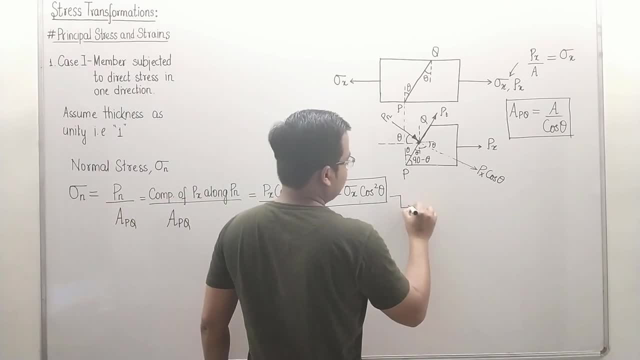 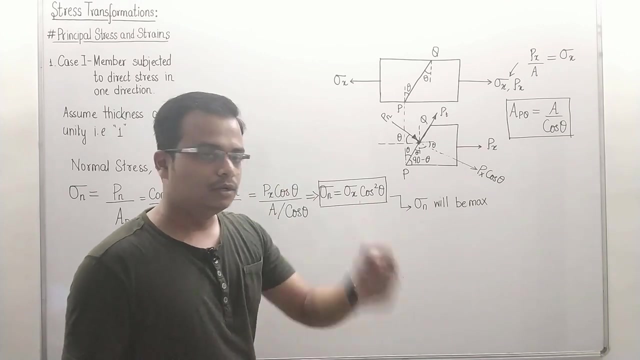 conclusion you can derive is that sigma n will be maximum for a particular value of theta. sigma n will be maximum when this cos square theta is maximum. and when is sigma x cos theta maximum? when theta is equal to 0 degrees. So maximum when theta is equal. 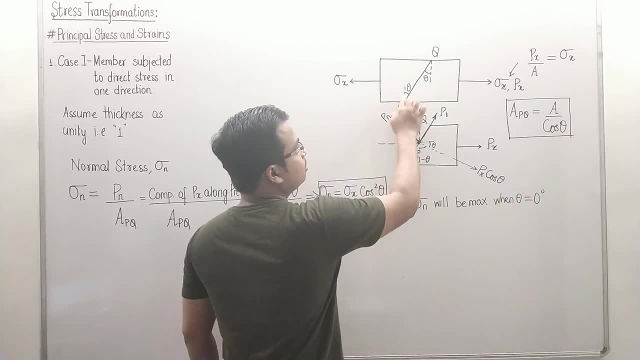 to 0 degrees, and when theta is equal to 0 degrees, this theta will be 0 degrees clockwise. we have taken the angle. then this oblique plane will become absolutely vertical. Okay, so again, this is the same result which we already know: normal stress will be maximum. 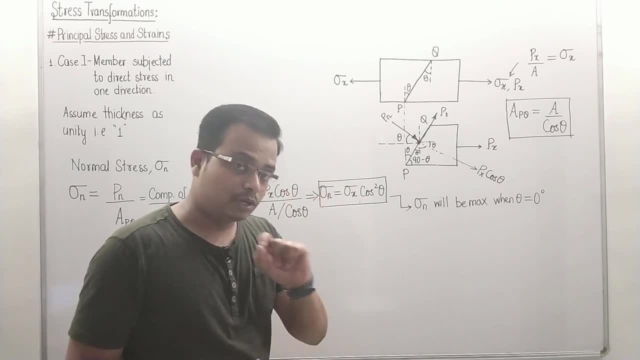 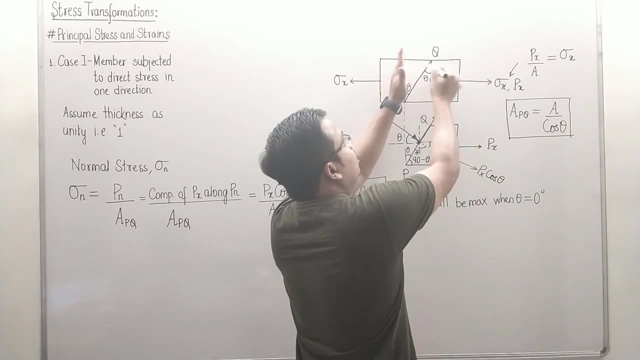 on a plane which is perpendicular to the axis. that is for sure. you can note this down. If theta is equal to zero, that means the plane is going to be absolutely vertical. Now, the absolutely vertical. like this, It will be perpendicular to the axis. Okay, So normal. 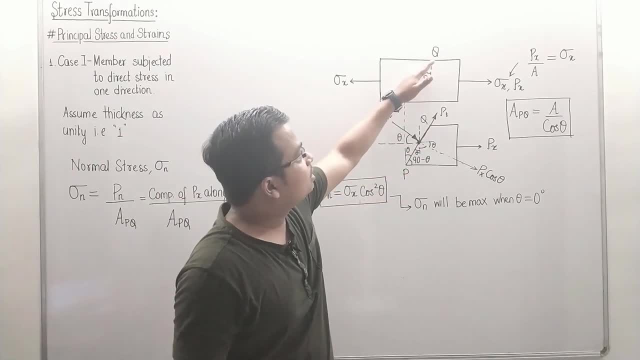 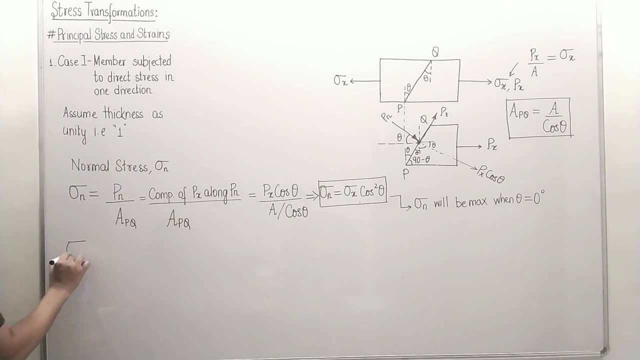 stress will be maximum when, when, the plane makes an angle of how much 90 degrees. That is it. That is the first result which we can write. Second thing is sigma t. This is the shear stress, by the way. So we are right now, we are representing this by sigma t. You can also: 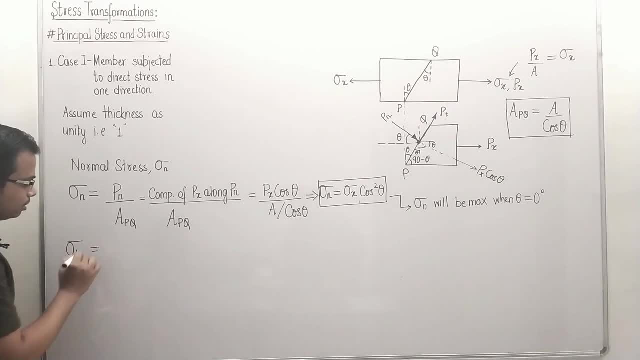 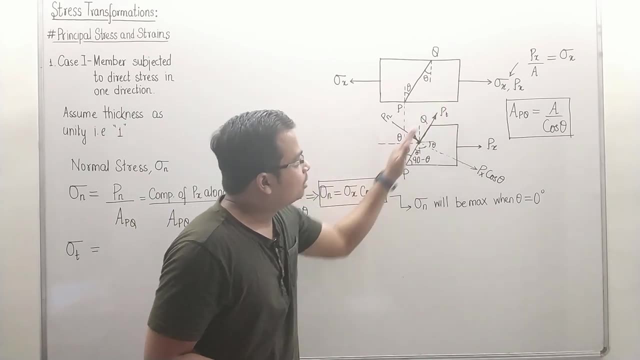 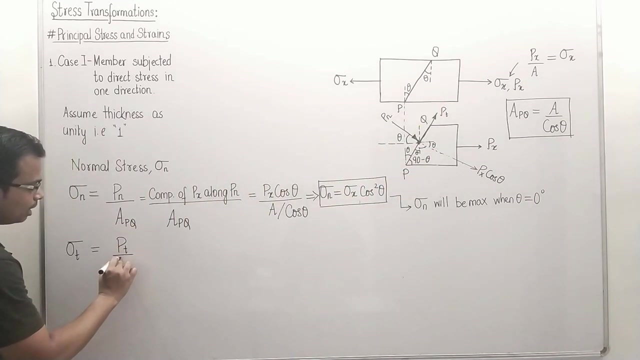 write this as simply tau. Okay, Because here, force along this plane on a direction, or should I say force along this tangential direction. with respect to the plane, this tangential direction will be taken into account. So this is a fairly simple. This is pt over again, apq. 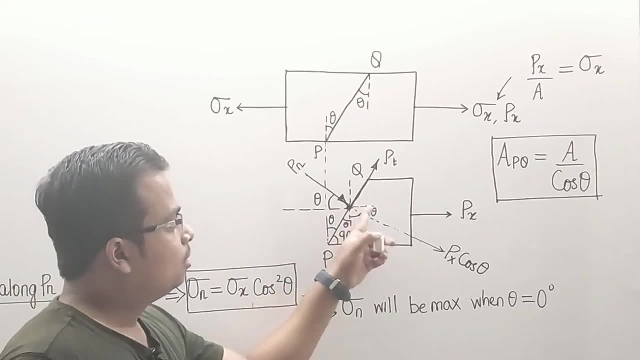 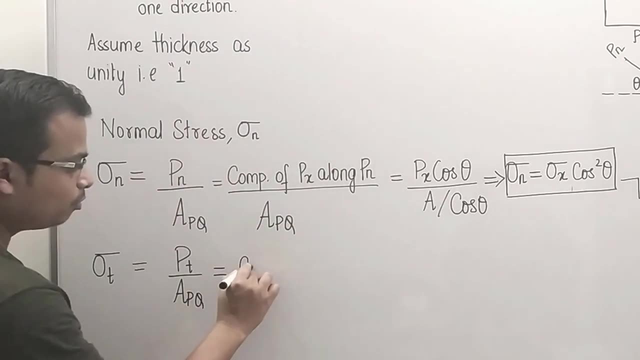 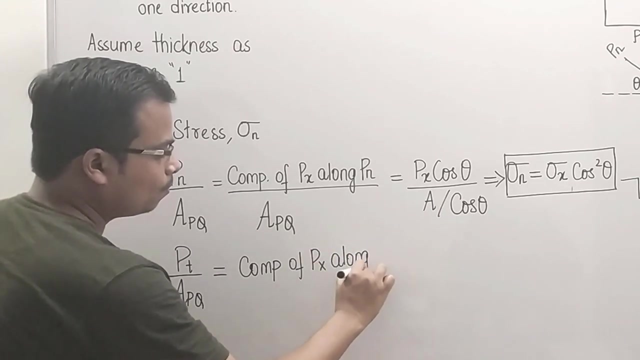 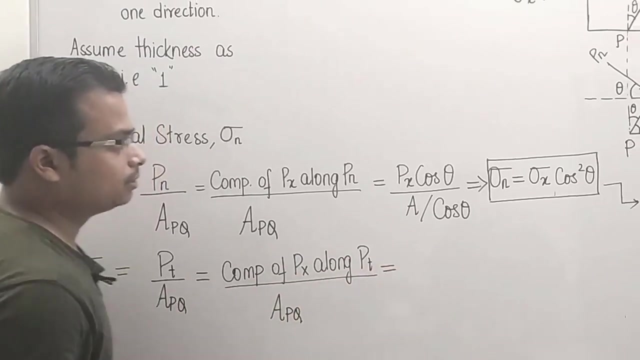 Now pt. if you watch here, that is, if this is px, Okay. Here we wrote component of px along pn, Okay. And here we are going to write component of px along pt. And all of this divided by well, it is quite basic apq. So, component of px, Component of 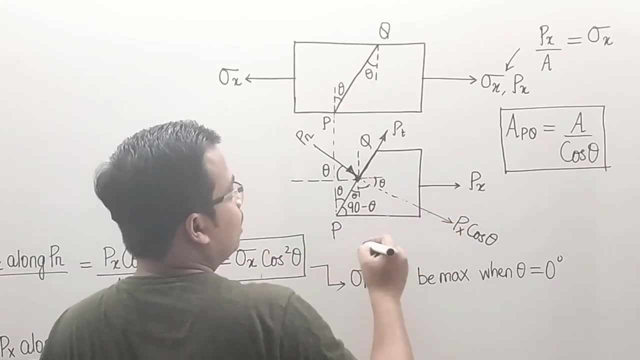 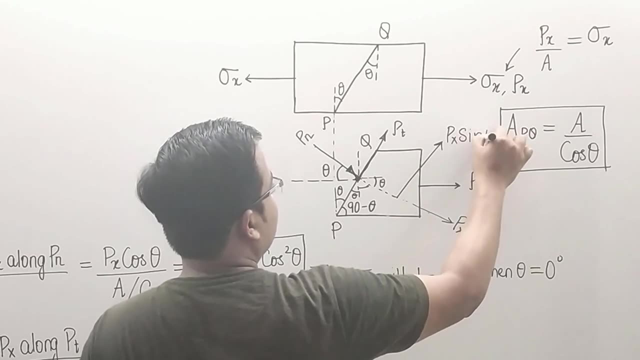 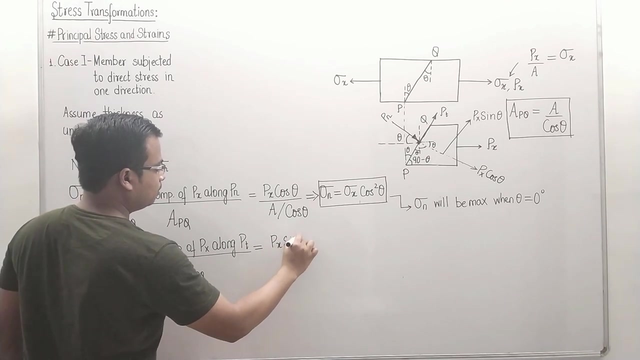 px. this was along pn and along pt. Well, along pt, the component of px is going to be this way. Well, that is px sine theta Done. That is it. So this is px sine theta Area. we know very well. 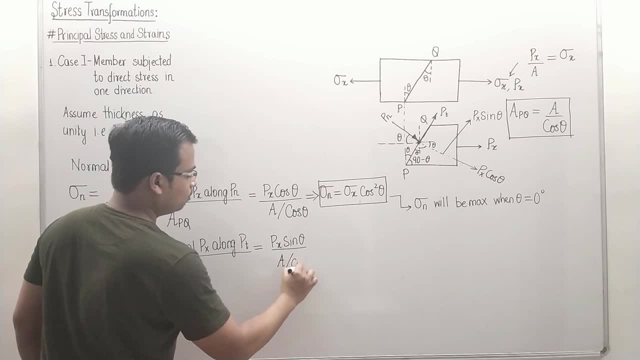 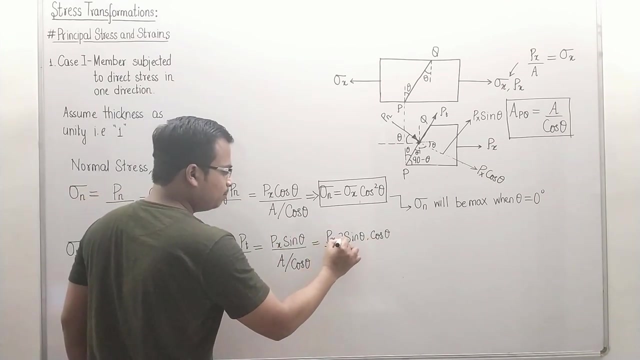 You already know this apq is nothing but a over Cosine theta. We just need to simplify this: px over a And this is sine theta, cos theta. What we need to do, try to use multiple angle formula, Multiply by 2 and divide by 2.. This. 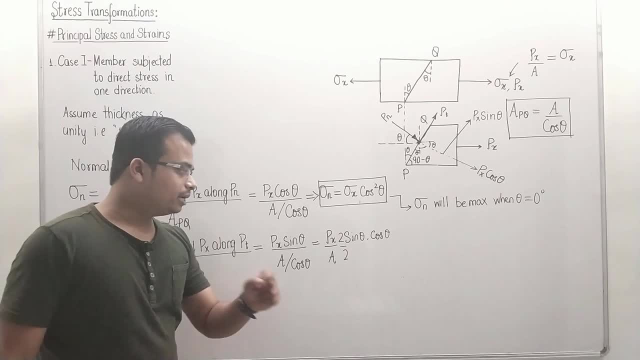 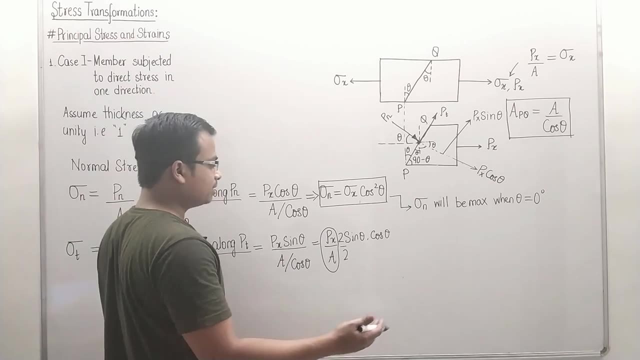 becomes 2 sine theta, cos theta, which is sine 2 theta. So there you go. This over here represents sigma, Sigma x, by the way, Actual tensile stress in the x direction. So there you have a final. 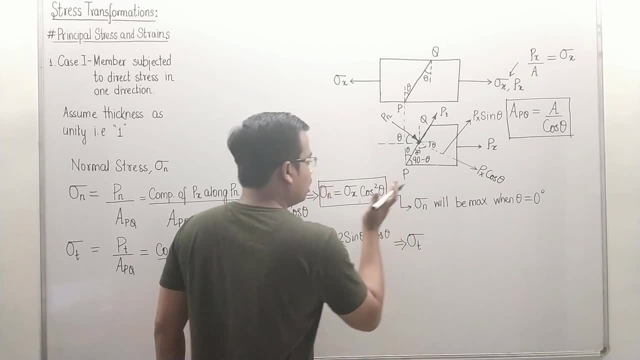 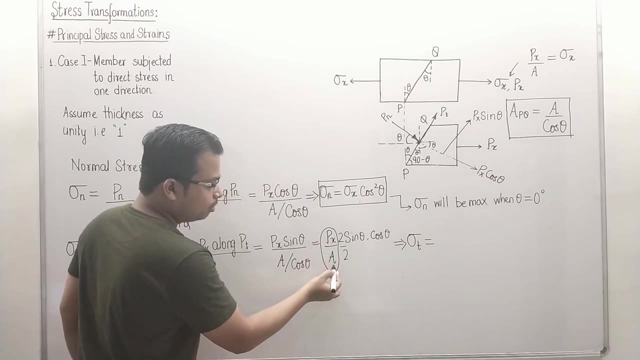 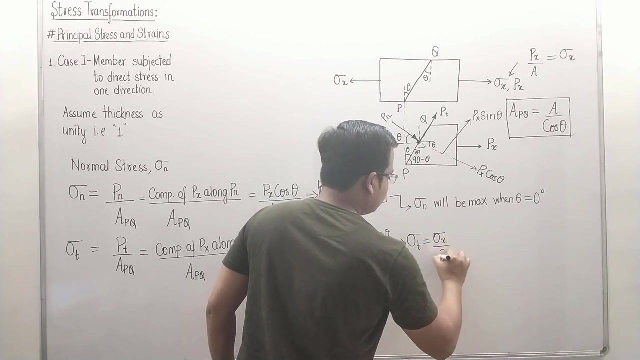 result: Sigma t or the shear stress along this oblique plane. Okay, Shear stress. Sigma t will be equal to what? Well, sigma by 2.. Let me just write this properly: Sigma x by 2, sine 2, theta Now. 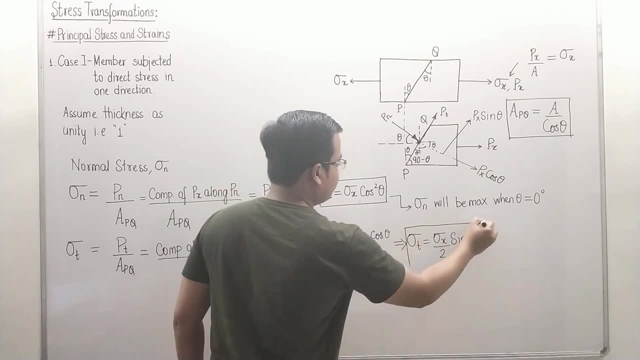 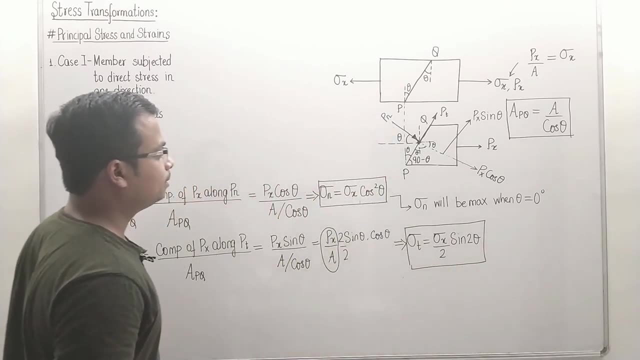 again. we need to think: When will we have a maximum value of shear stress? Okay, So tau t. where shall I write? There is absolutely no space. Okay, Let me just write it. So write it over here. 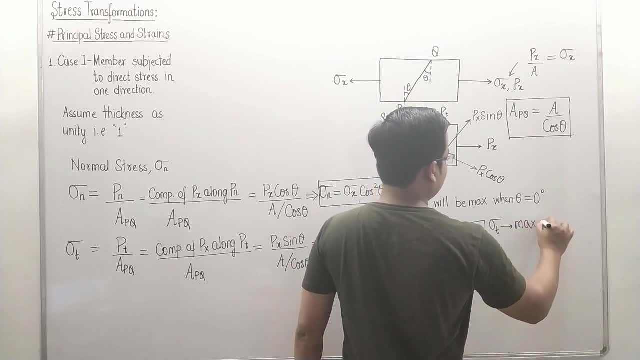 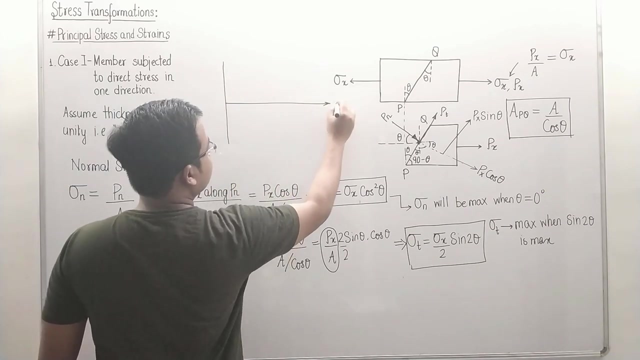 Tau t is maximum. When Sine 2 theta is maximum. Sine 2 theta is maximum. So just take a look at this sinusoidal curve. I am pretty much sure that you must have seen this. This is, let's say, 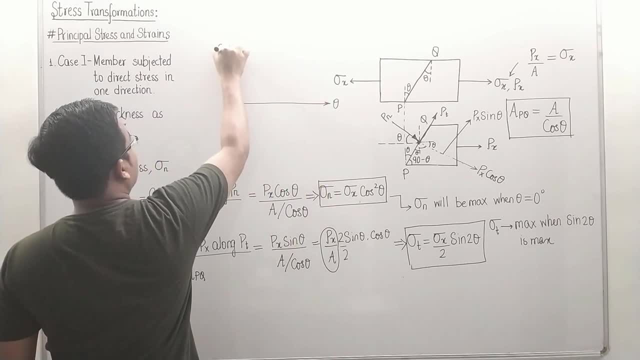 this is theta, And let's say this is sine theta. So sinusoidal curve, something like this, Isn't it Over? here we have the maximum value. Okay, So the maximum values are obtained at two different points. One is plus 1, one is minus 1.. This over here. 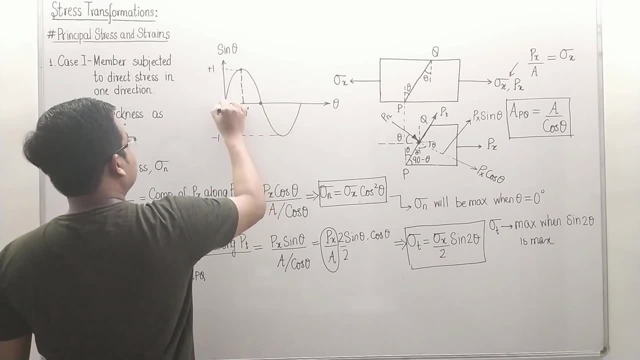 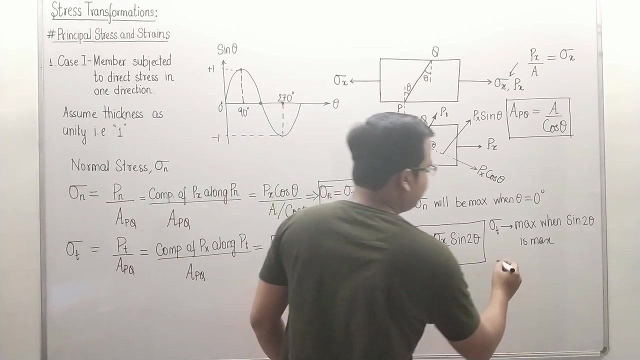 is corresponding to 90 degrees, This is 180.. This is 0 degrees And this over here is for 270 degrees. That means the value will be maximum when 2 theta is equal to 90, when 2 theta is equal to 270, which is quite clear. So this is the maximum value. So this is the maximum value. So this is. 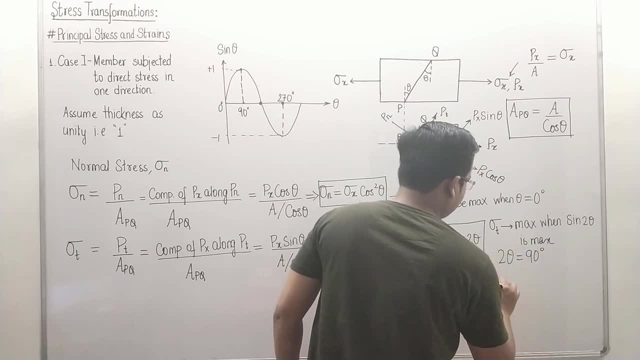 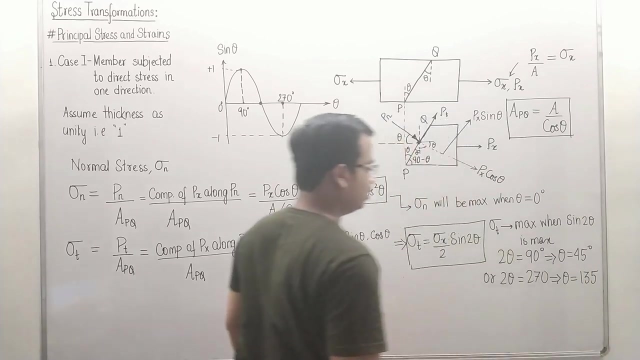 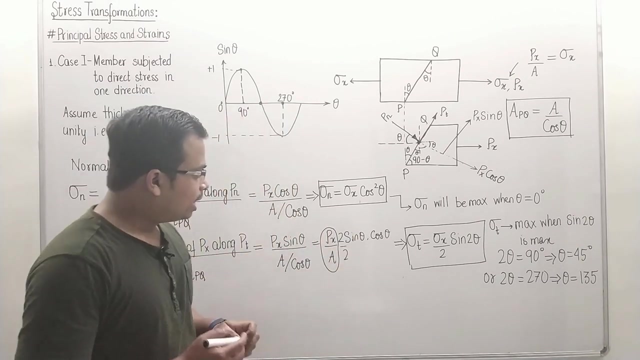 you just have to do the math. Theta is going to be equal to what? 45 degrees, And this theta is going to work out as half of 270. That is, 135 degrees. That means there are two planes which depict the value of shear stress maximum, And let me just show that those two planes are essentially 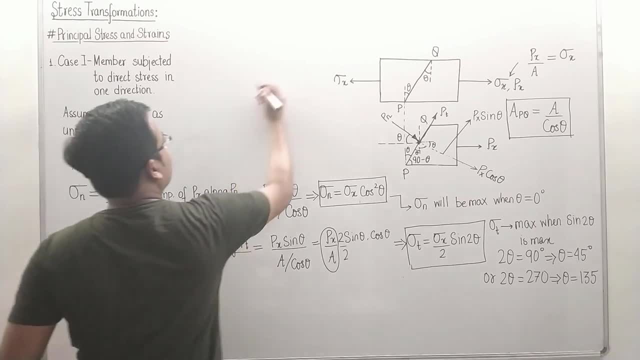 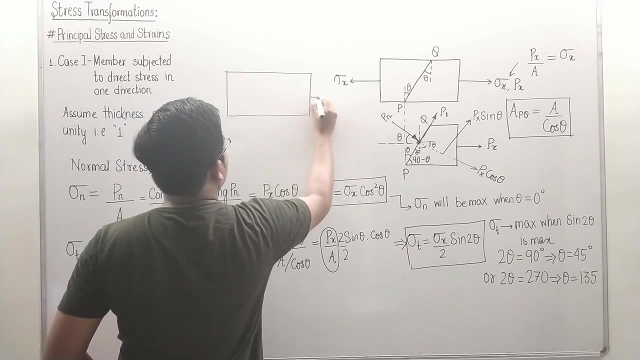 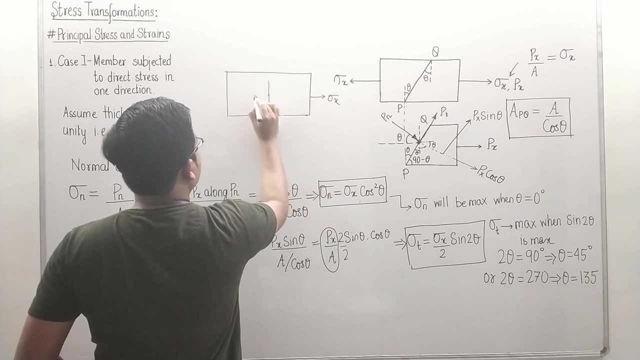 Like this. it's fairly simple. Okay, here it is. That's the member, Okay, subjected to an axial loading in the x direction. Okay, forget about this. now Let me just make a coordinate axis. Okay, here the angle measurement was done in the sort of clockwise sense from. 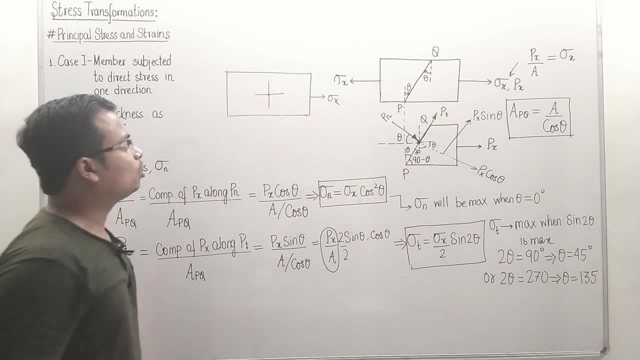 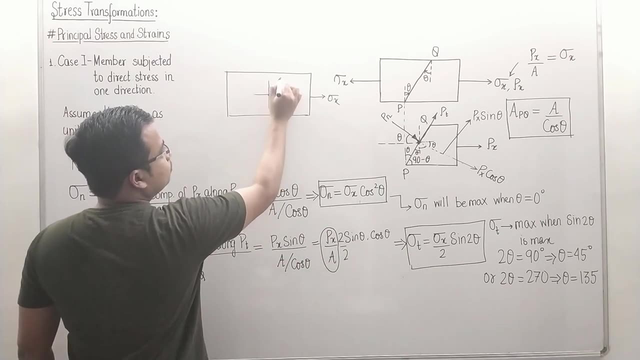 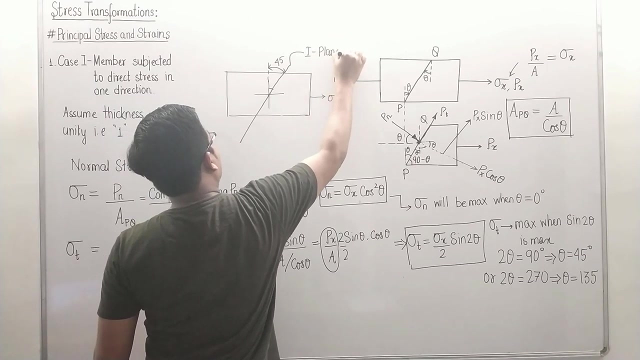 here, from here with the vertical. So here also we are going to do in the clockwise sense with the vertical, from the vertical. only How much? 45 degrees. So 45 degrees, That's it. Okay. so this angle over here is 45 degrees And this represents the first plane of shear. 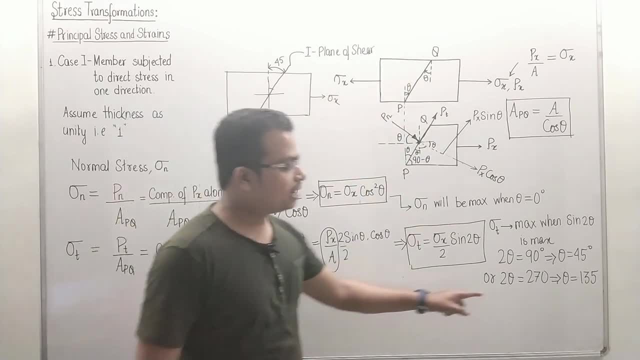 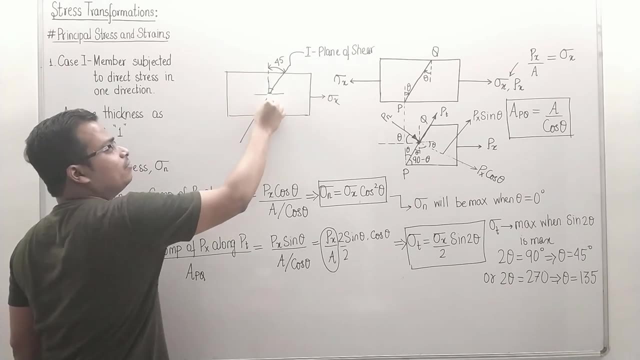 Let me just show you the second plane of shear that will be obtained at an angle of 135 degrees. So starting from here, zero, 90, and this is 180.. So between 90 and 180, there is going to be this and extend this. 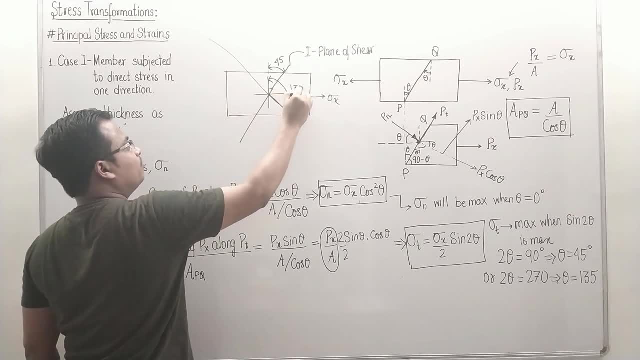 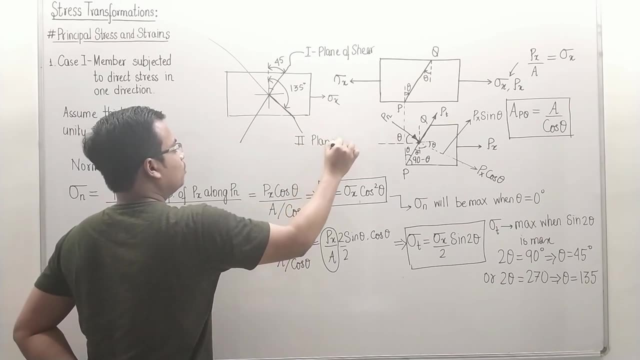 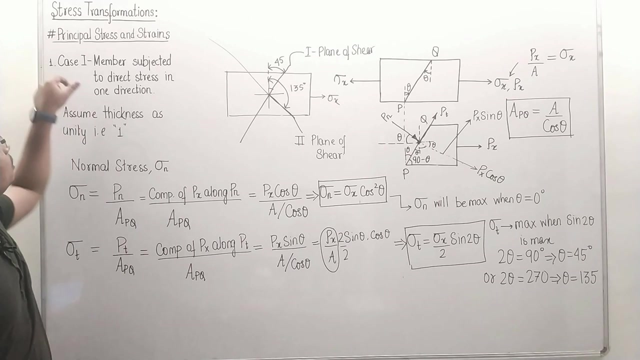 This angle over here, guys, is going to be equal to 135 degrees, And this over here is the second plane of shear. So that's all you have to know about this case one when a member is subjected to a direct stress in the x direction. 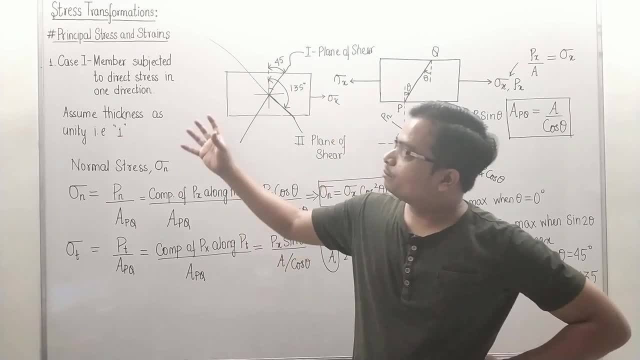 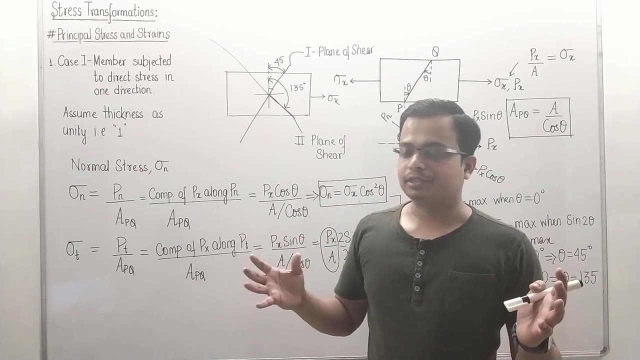 Now, in the next case I will be talking about a member subjected to two mutually perpendicular stresses. then we'll also take cases that is based on pure shear, and then case four is a combination of case two and case three. Okay, there are going to be two mutually perpendicular 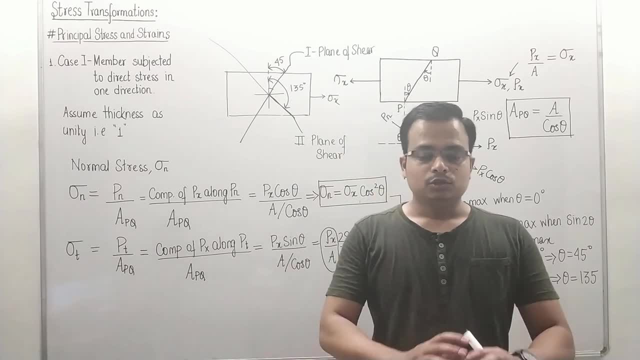 stresses accompanied with a shear stress. So, guys, that was all for today. I'll see you again in the next video. Until then, take care, Have a nice day, Keep learning, Thanks.